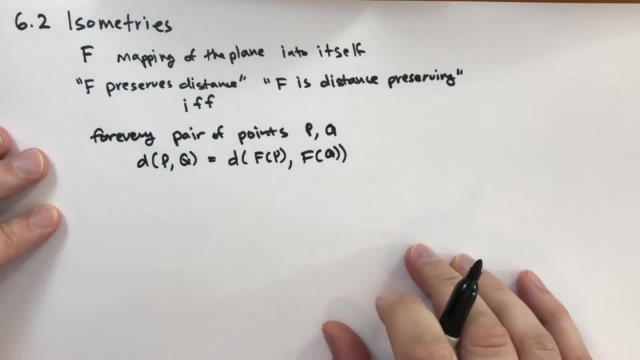 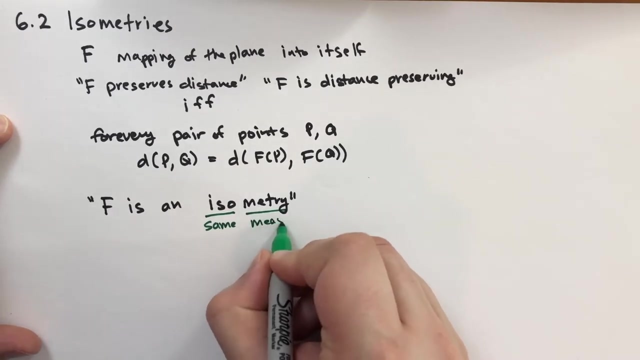 So those two distances are equal if F preserves distance or F is distance preserving, And so we say F is an isometry. when this is case, This is the case. So isometry is a useful word. It comes from Greek. Iso means same and metri means measure, So the measure of the distance is the same under the 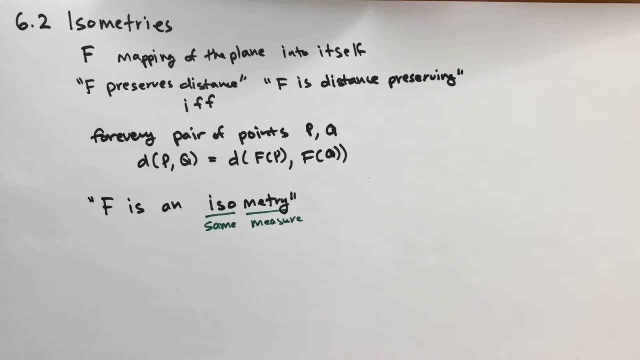 mapping F: All right, pretty simple stuff. It's not that terribly complicated. So we're going to be dealing with mappings that do isometry, some mappings that don't. All right, so the following are distance preserving. So these are isometries. 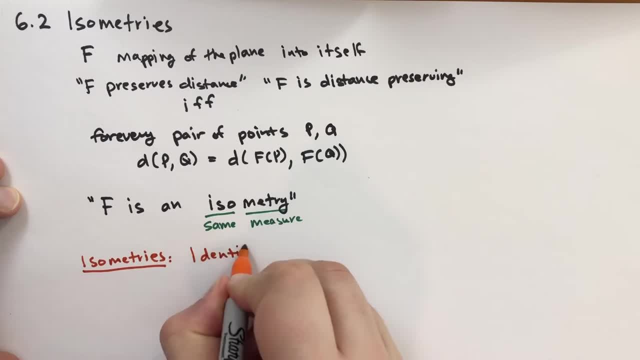 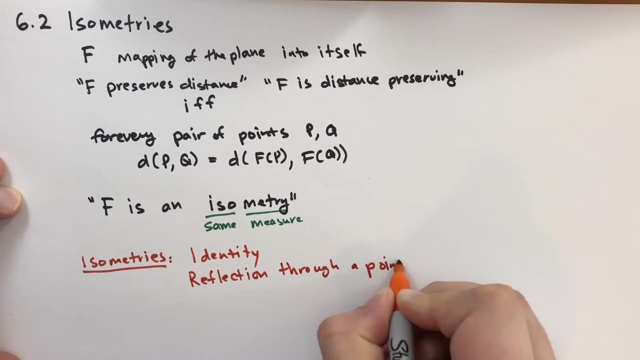 We have the identity. of course It's not listed in the book, but it's pretty trivial to understand why that is. Every point maps to itself, so the distance between the points will always be the same: Reflections through a point and reflection through a line. 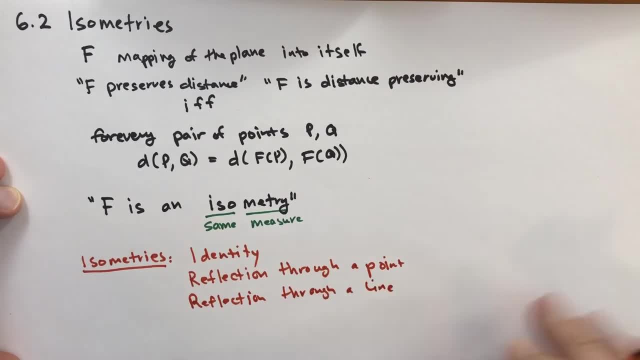 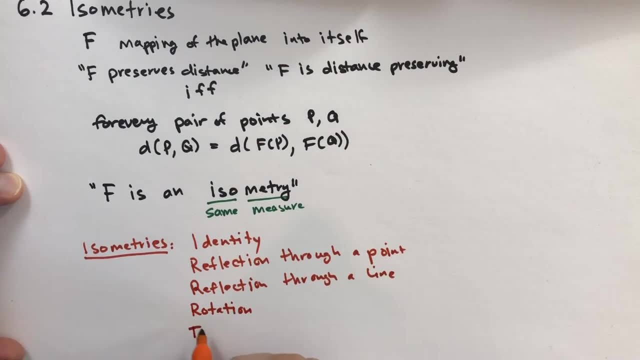 And we have rotation And finally, we have translation. These are all distance preserving isometries. This is not the complete set of all possible distance preserving mappings or isometries. This is some examples of mappings that you already know about that are distance preserving. In fact, we can compose these. 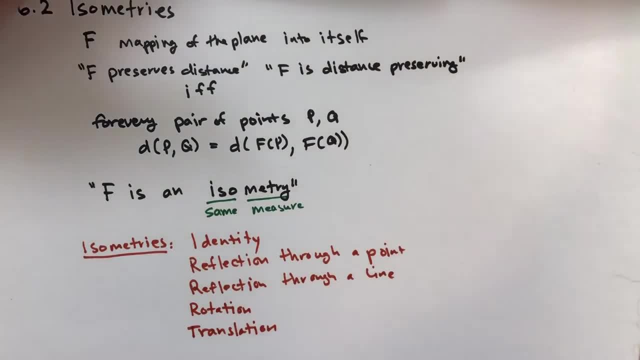 into new, new isometries, into new mappings that are also isometries. we'll talk more about that in the next section, section three. uh, and we're not going to prove that these are the case, we're just going to assume them and we're going to talk about the implications of these guys. but when we get into 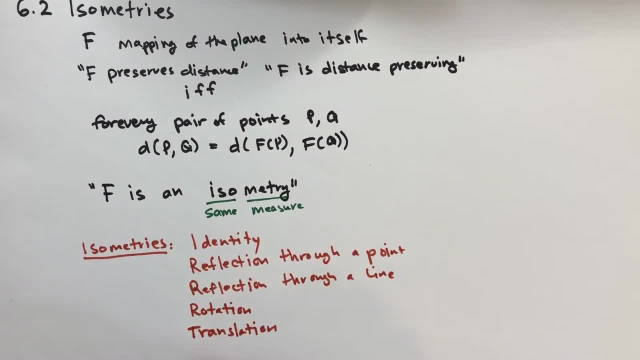 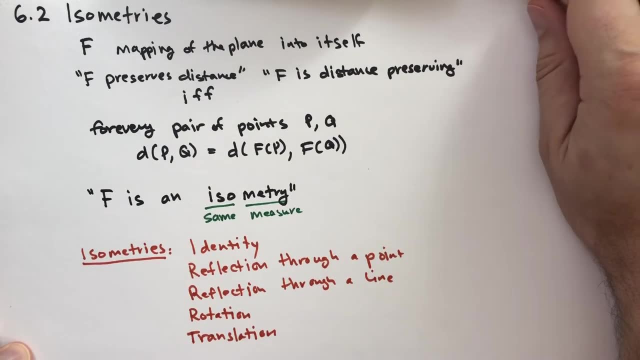 i believe section five- when we can start to numerically analyze geometry, we'll be able to prove these things using some a little bit of algebra and a little bit of geometry. all right, so here is an interesting remark about isometries. we're going to learn interesting properties about. 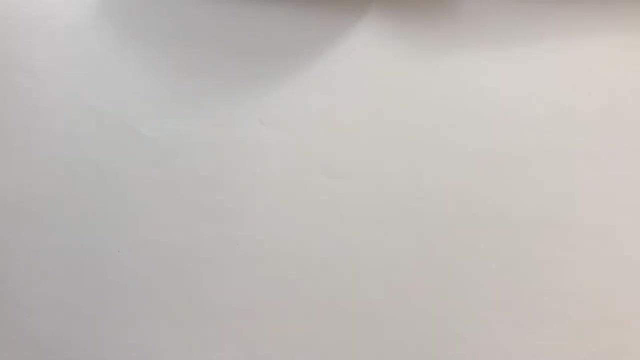 isometries. we're going to use those properties to prove some things and we're going to do some interesting things with it. this is basically the modus operandi, mo of mathematics. so remark: so f is an isometry. let's say: okay, so we have f. that's an isometry if p and q are distinct points. 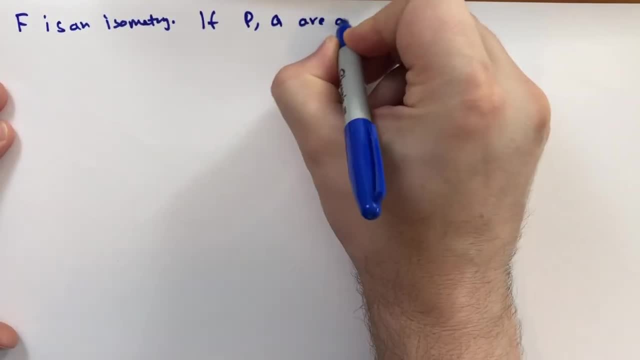 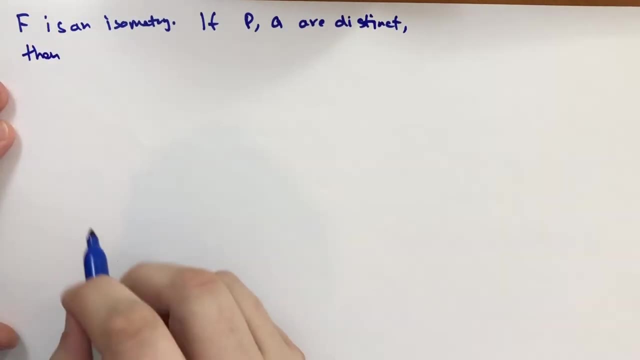 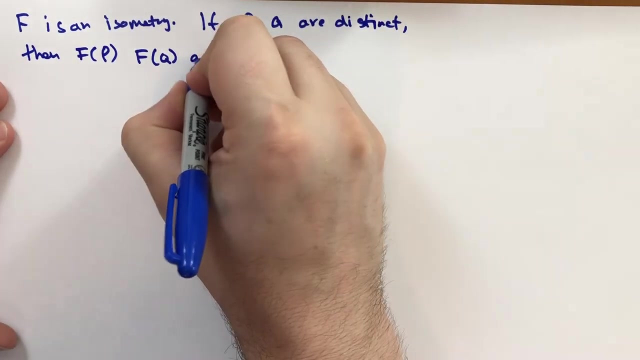 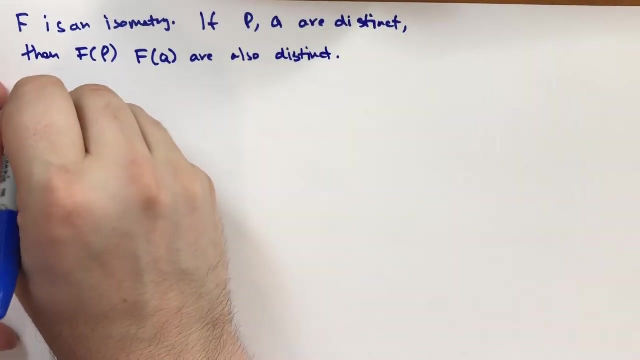 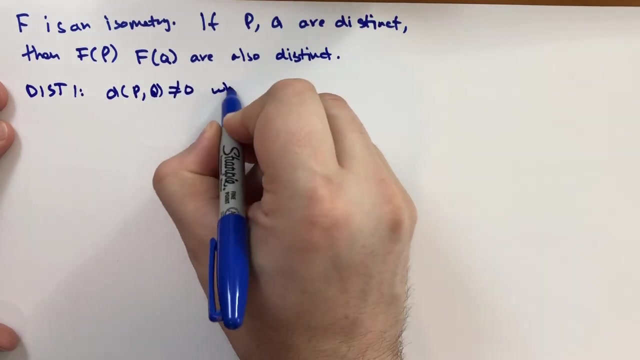 are distinct, that means the distance between them is not zero. if they're distinct, then f and p and f and q are also distinct. Why is that? Because, using the property dist1, if you recall, dist1 says that the distance between p and q is not zero when p is not q And the distance between p and q is zero. 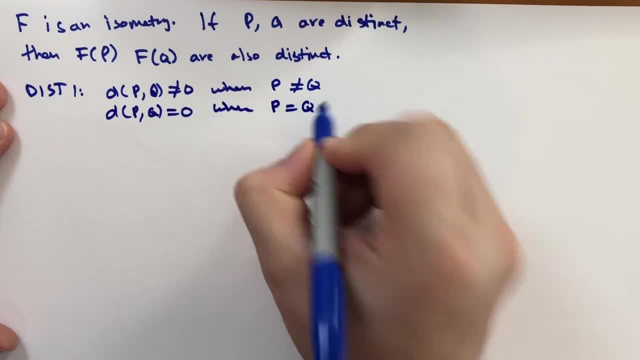 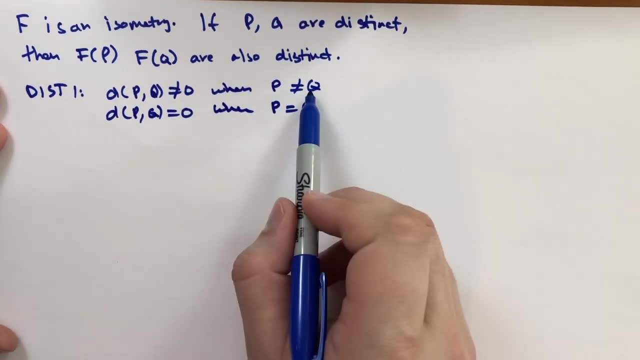 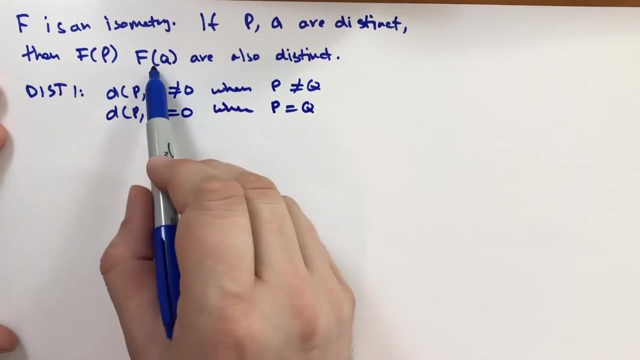 when p and q are the same points. So if we have a distance between p and q because they're distinct, they're not the same points, so the distance is not zero. So if f is an isometry, then the distance between the mapped points f and p, f of p and f of q will also. 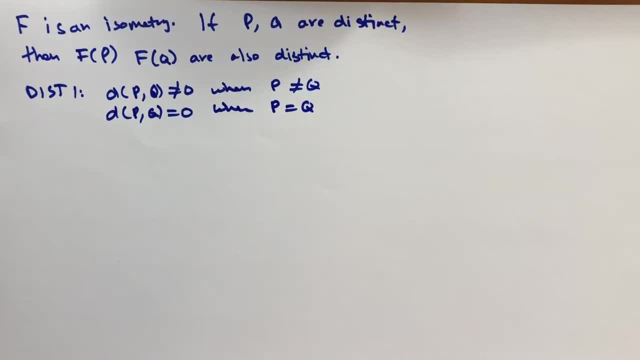 have a distance between them, and so they will not be distinct. Fairly simple observation. It's going to be useful, And we're going to do this again and again throughout this section. We're going to talk now about what happens when you map a set of points, And this is: 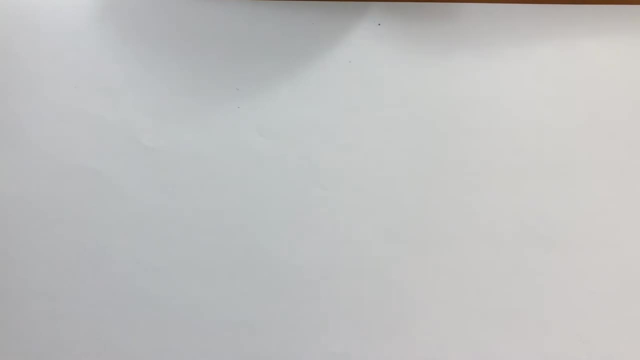 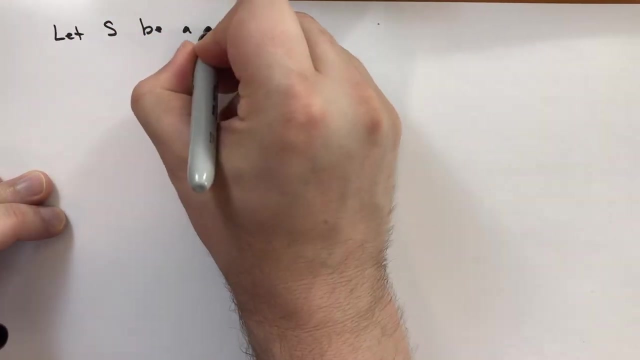 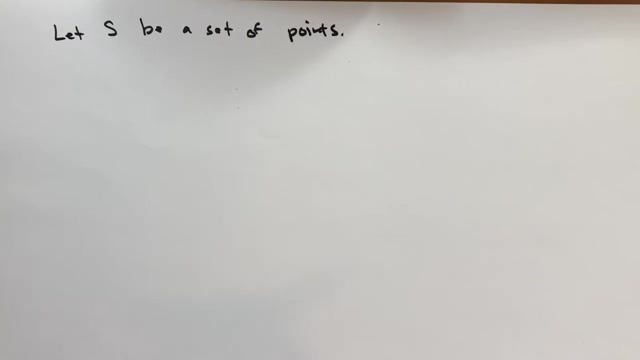 going to be important because we want to do things like mapping segments and circles and things like that. So let s be a set of points. So this could be just a random collection of distinct points, or it could be like a line segment, it could be a triangle, it could be the area inside of the triangle, any one. 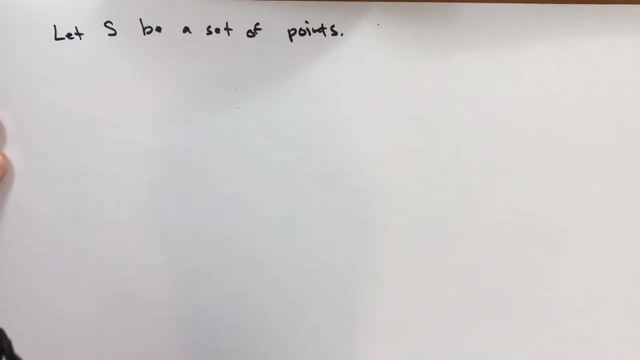 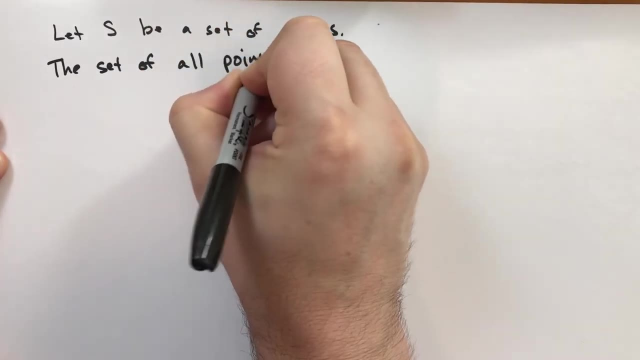 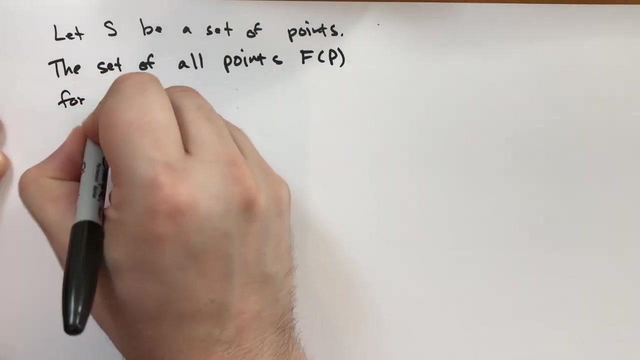 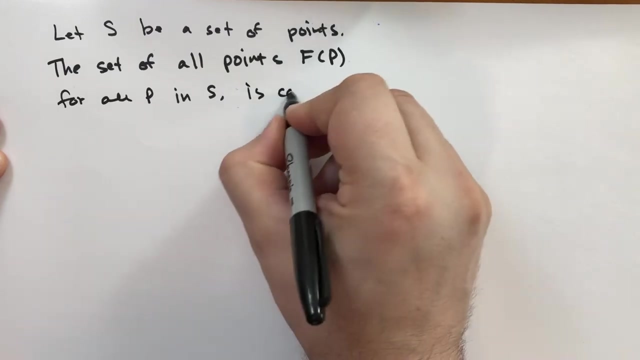 of those kinds of things. that's a set of points, Okay, So the set of points, of all points, where you take each of those points and map them through, f, okay, For all points. p and s is called the image of s. 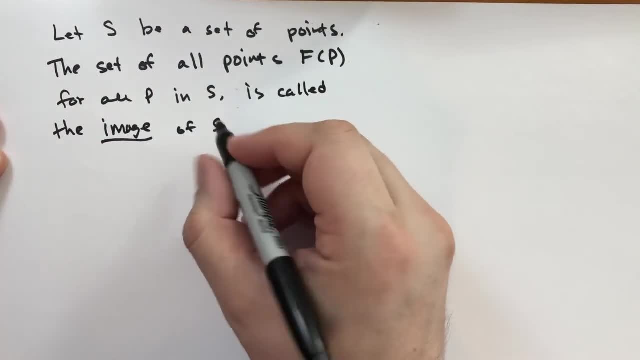 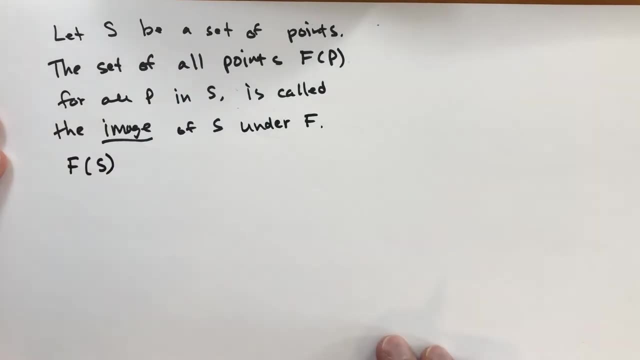 Image of s through f under f And we say f of s. Okay, That's how we denote that. So this is different than what we're used to, because normally we put a single point in there, but now we're actually putting sets of points through. 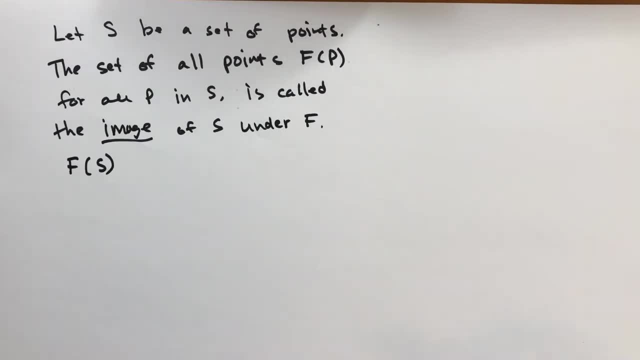 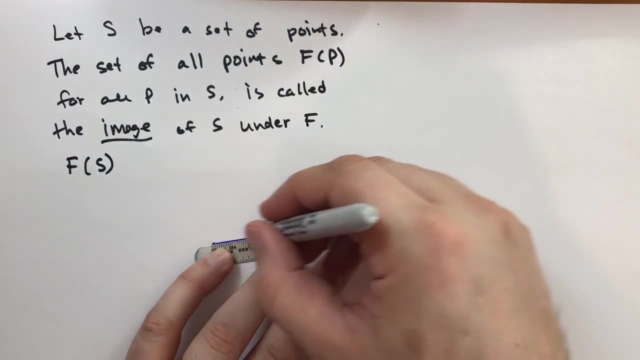 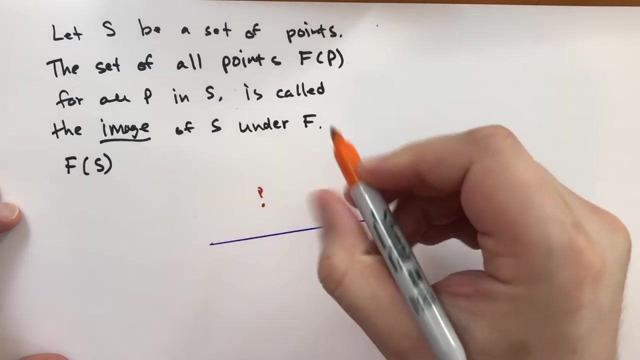 And we get a mapping of those sets of points. So we call that the image. So let's take, for instance, let's take a line, use my trusty dusty ruler here. So here's a line, and we are going to take a point p in orange, here a point p, and let's take a point q, and let's 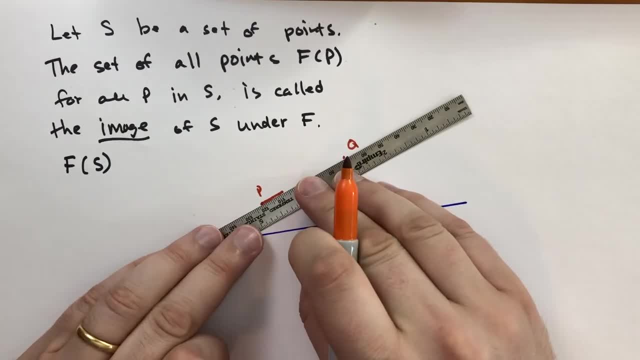 draw a line segment. Oh, I should use a ruler, so it's a straight line. Let's draw a line segment between p and q, And this is called p q bar right, p q bar, p q bar p. 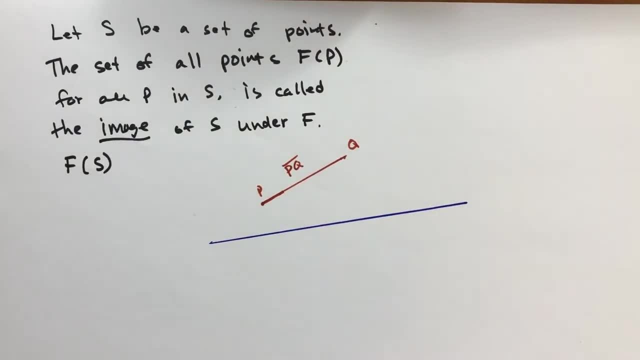 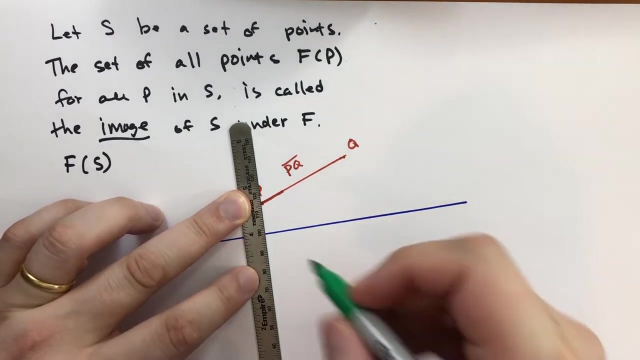 q bar. Let's do a line segment. So if we were to map all of these points, we would also get another line segment. Let's go ahead and try to find a perpendicular. Let's see that's about. let's start at 100.. 100. That's about 113, 116 actually. So let's go down right. 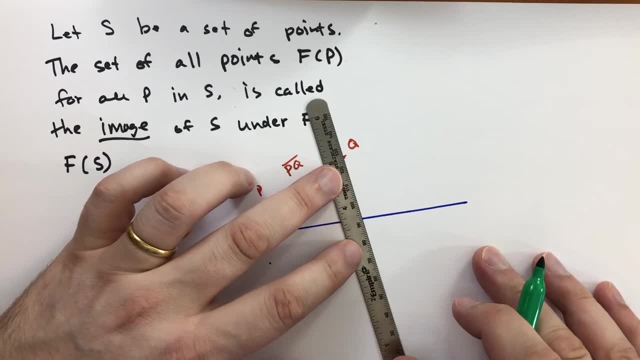 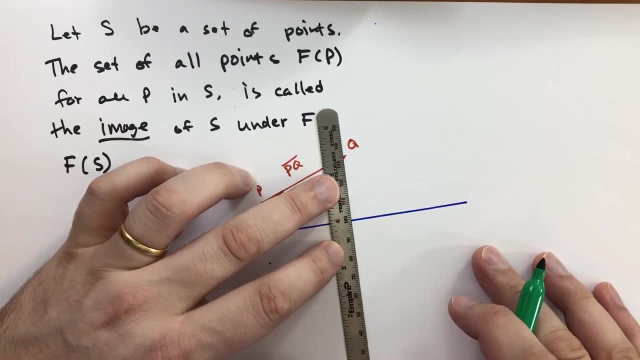 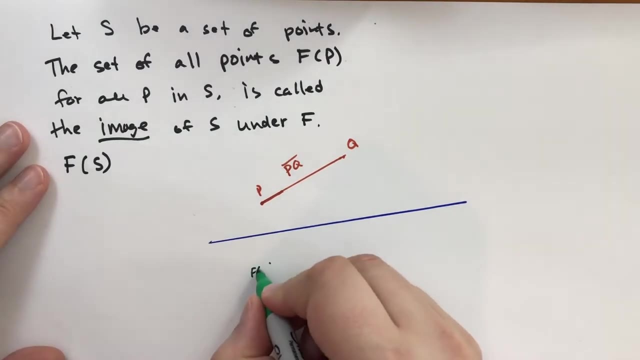 here And let's do another perpendicular to that point. The perpendicular would be perpendicular to the line. There we go and we start at 100. And that is up there at 135.. So we're going to have to go down 35,, 10,, 20,, 30,, 5.. And that's going to be. this is f of p, This. 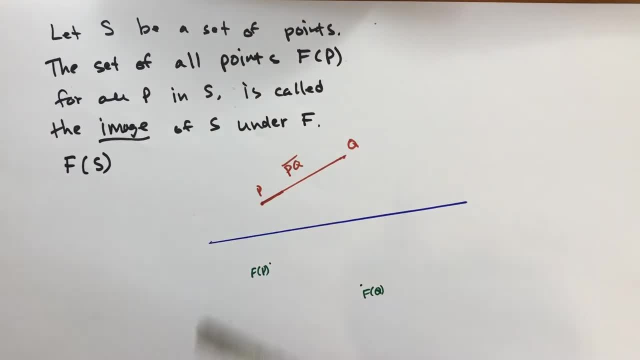 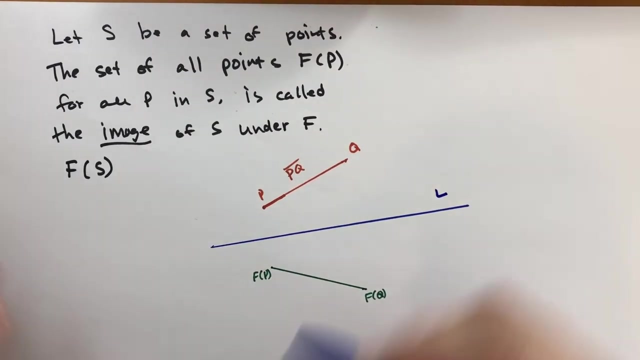 is f of q. Remember. f is the reflection through the line l. Did I give line l a name? I did not. Let's give l a name There. this is l okay, And so you can take each of these points. 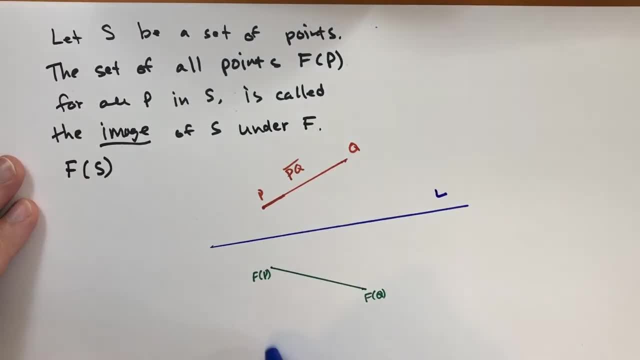 and you can map them and you'll get a line segment on the other end. So this, this thing here, if we call this pqs, okay, then this thing down here, this is f of the line segment pq, which is also equal to f of s. okay, So you can take and map single points like p. 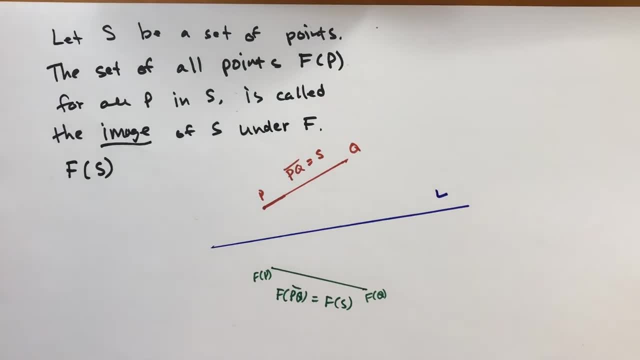 and q, and you can map entire sets of points as well. okay, And we actually note that here this is equal to the line segment that starts from p mapped through f and q mapped through f. It's that giant line segment there. This notation might be a little confusing. 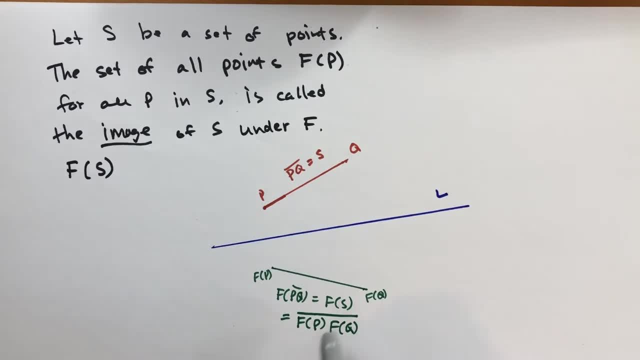 so take some time, if you need to, and think about what the different symbols mean. So this f of p is the point p mapped through f. This f of q is the point q mapped through f. this bar over the top says this line segment between those two points. so it's that green line. 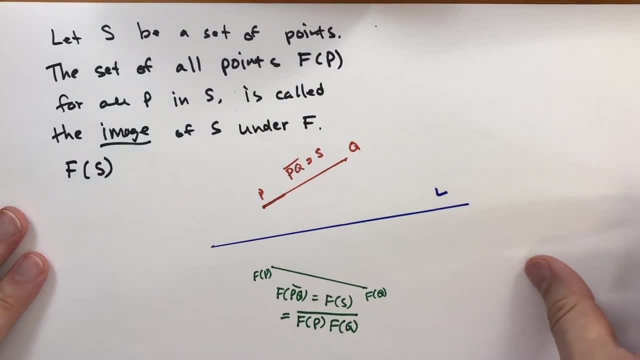 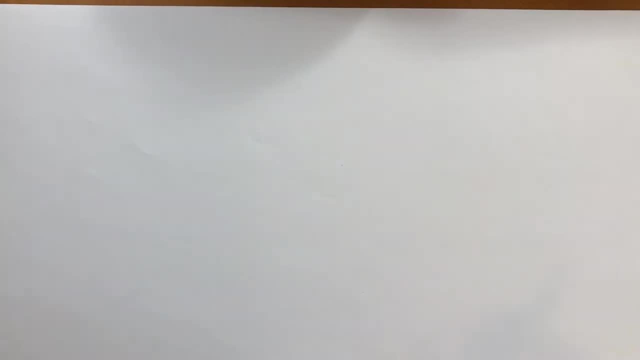 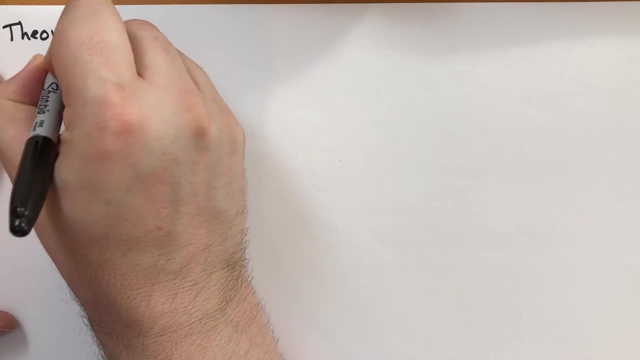 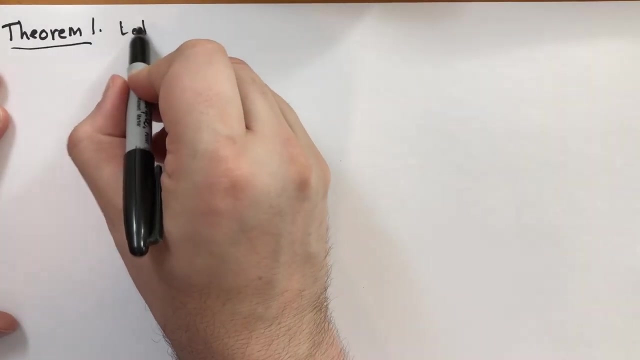 right there, all right, all right. now we're going to talk about some theorems. so, remember, theorems are things that we- um, we try to prove using the assumptions that we already have. so this is theorem one of section six two. i believe we're in six two. i hope we're in six two. if we're not, then i made a. 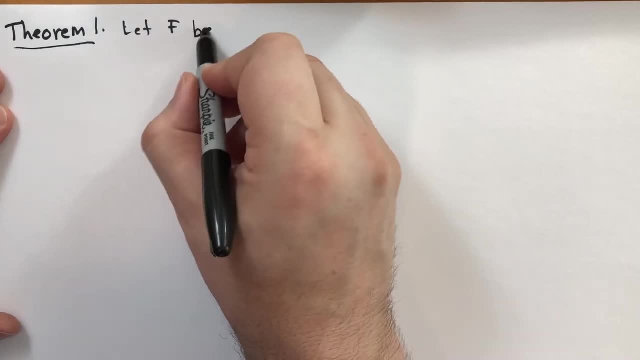 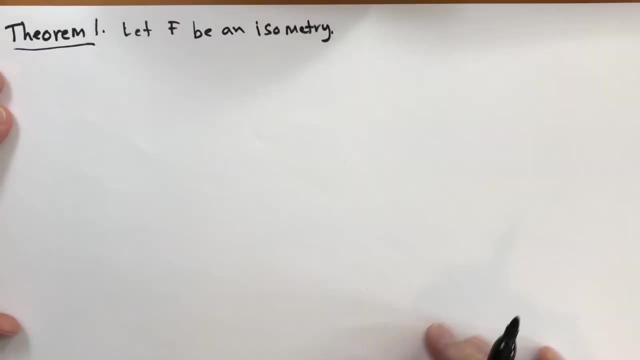 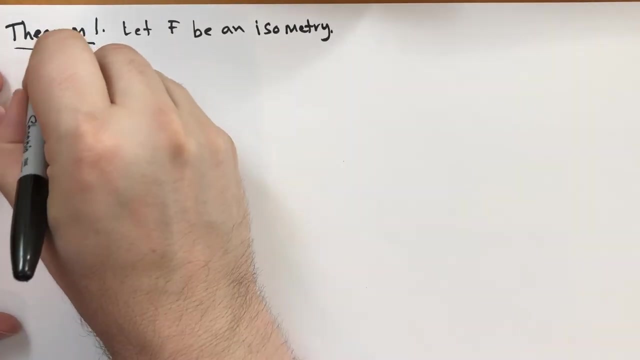 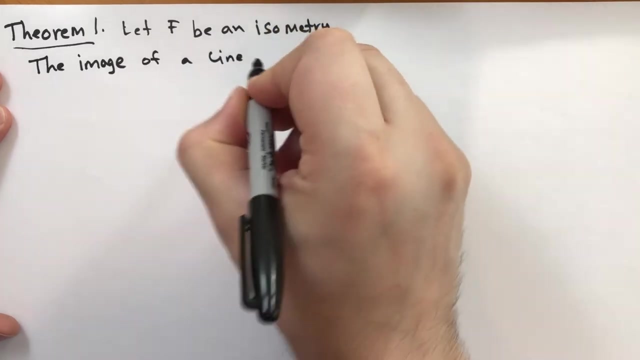 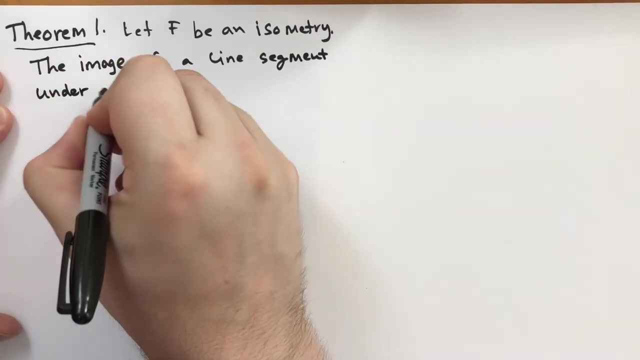 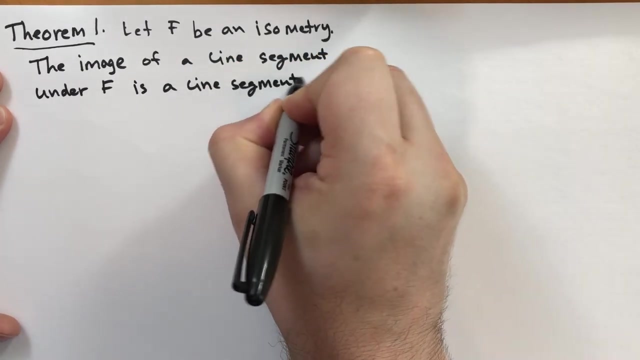 b and isometry. we've already defined that isometry. that's a mapping from the plane into itself that preserves distance right. the image of a line segment under f is a line segment, all right. so when we take a line segment and project it through an isometry, we get 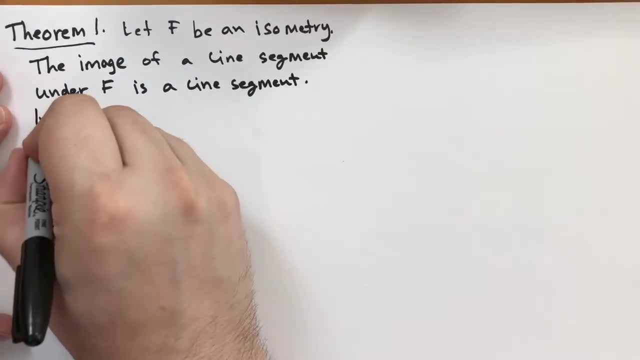 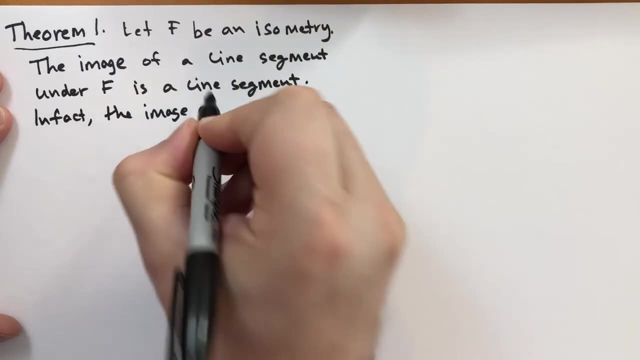 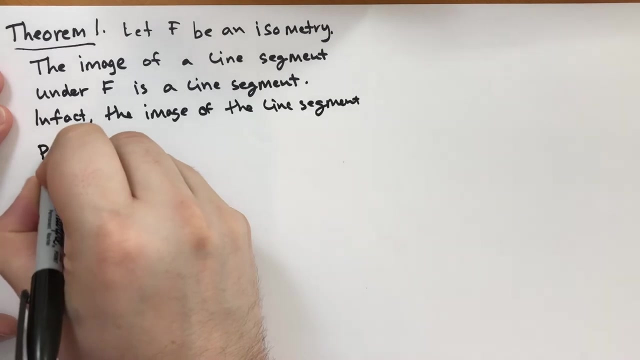 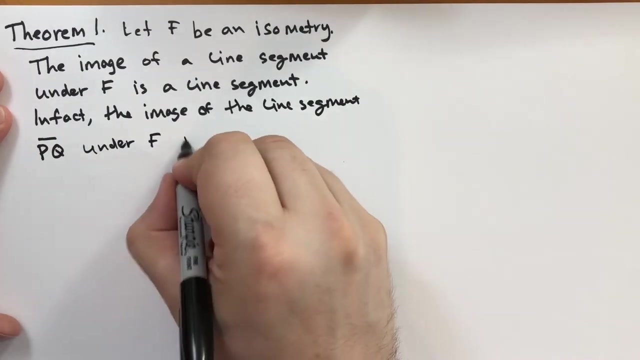 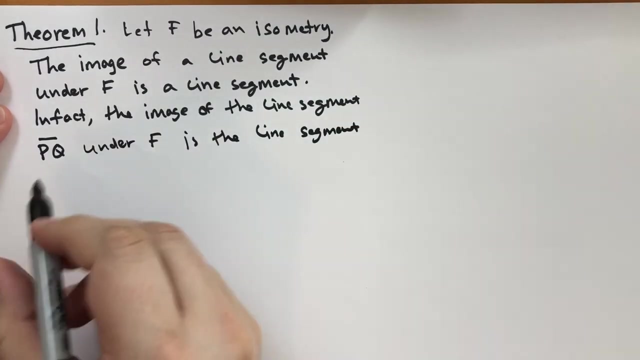 a line segment. in fact, the image of the line segment pq bar under f is the line segment between f of p and f of q. oh, let's add an extra e there. f applied to p and f applied to q. okay, so that's the theorem we're. 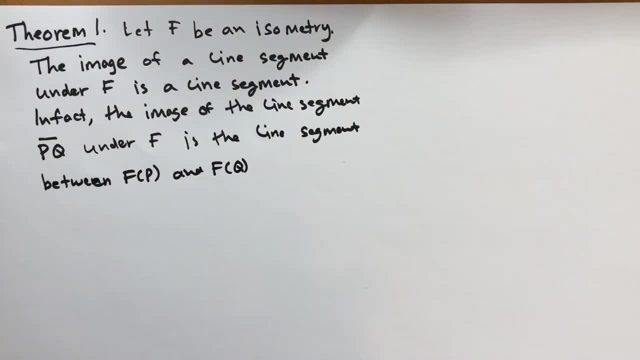 going to try to prove this. now, this proof is going to be a little different because we need to prove it not just for some points, but for every single point on that line segment. so we need to be able to walk through and find each point and then map them and show that they end up on the line segment. 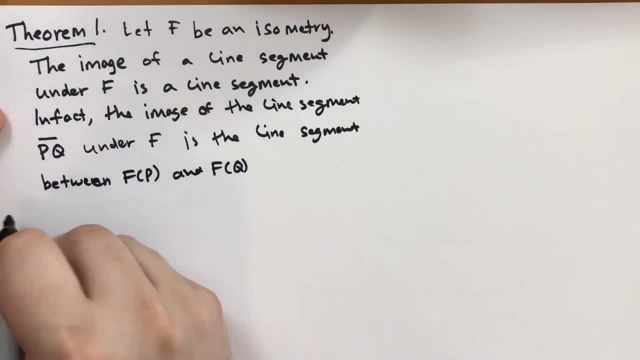 that we described here. so, in order to prove this, in order to prove this, first we're going to do it for one point, we're gonna do it for one point, then second, we'll do it for all points. okay, so pay attention, here, this is going to go a little bit quick. 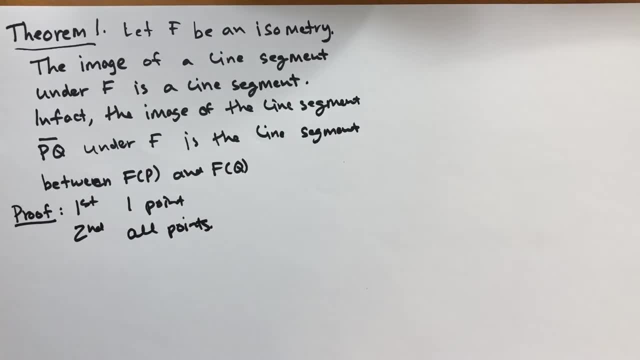 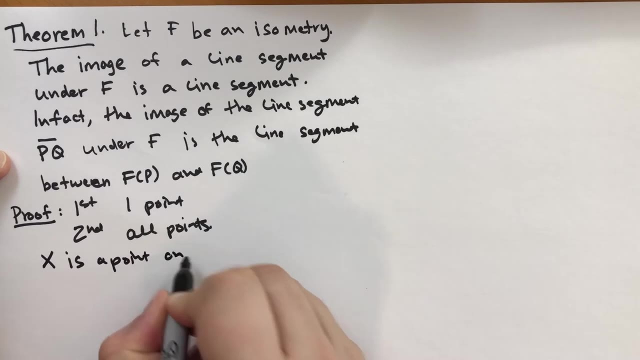 uh, this is on page 145 in the textbook and uh it there's a lot of texture, but it's kind of simple. the idea is simple. okay, so the proof. so let x be a point on pq. so x is a point on pq. okay, so it's one of these points on that line segment. 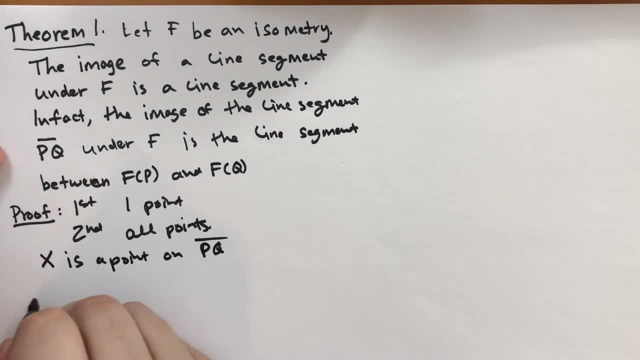 okay, so we denote f of x. x prime is equal to f of x and we're going to use p prime is equal to f applied to p and q prime is f applied to q. okay, And that's just going to make it a little easier. 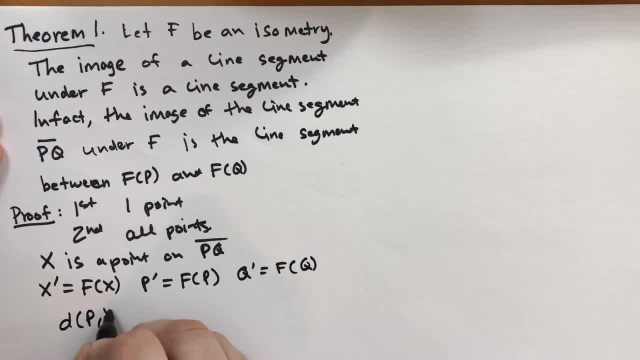 to write things down. So we know that the distance from p to x is equal to the distance from p prime to x prime. Why is that? Because we're dealing with an isometry here. And likewise the distance from x to q is equal to the distance from x prime to q prime. Again, we're dealing with an isometry. 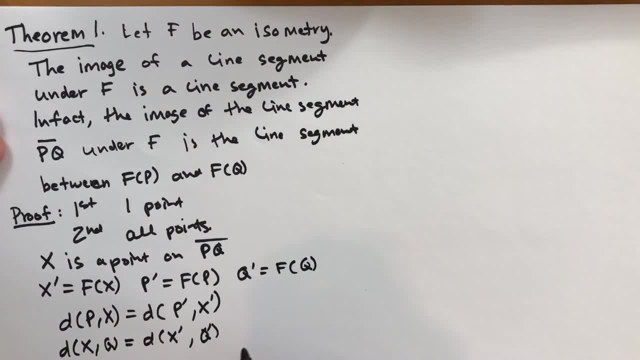 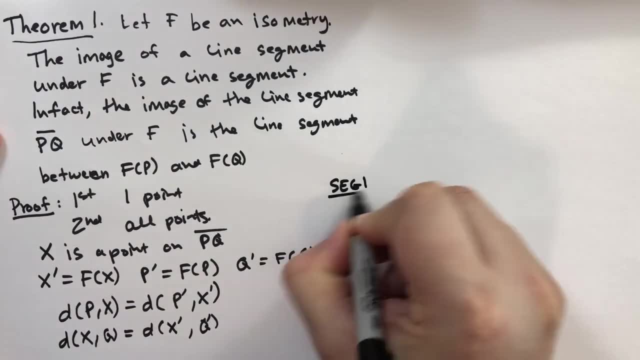 here. okay, Using the theorem seg1, we know, is this on the map There? it is okay. So using seg1, if you go back and review that seg1 talks about how, if the distance, it says that the distance 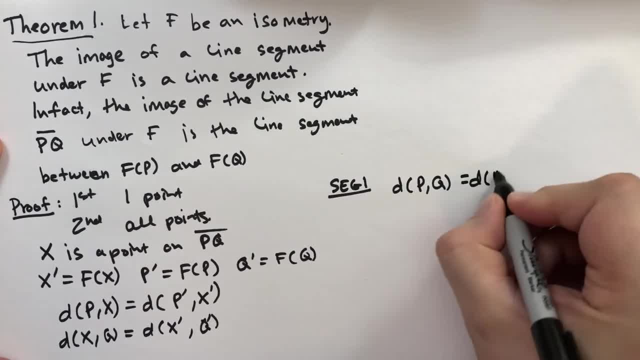 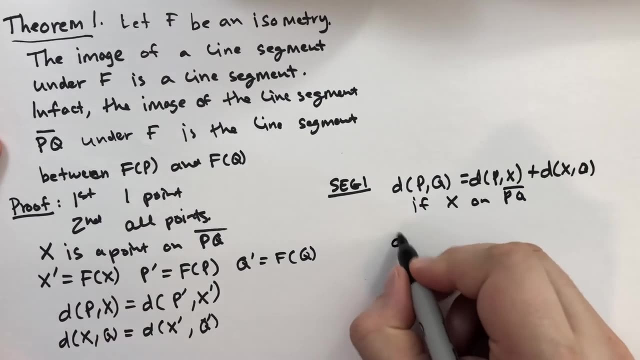 between p and q is equal to the distance between p and x, added to the distance from x to q. if x is on pq, okay, That'll pq line segment, all right. So, substituting things in, we get the distance from p prime to q prime, which is the same as. the distance from p to q is the same as. 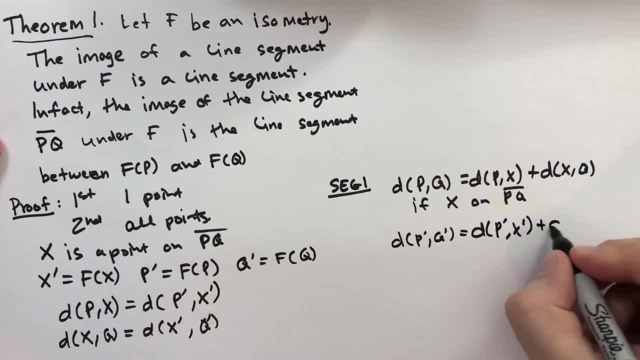 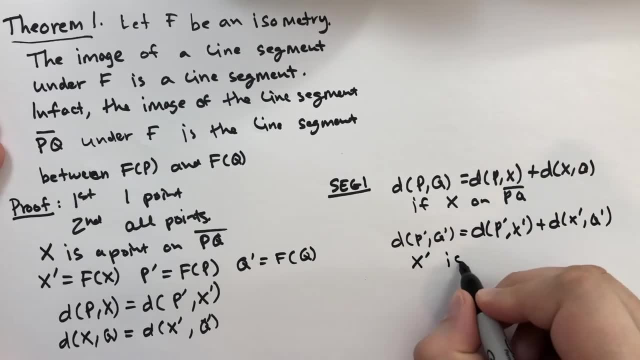 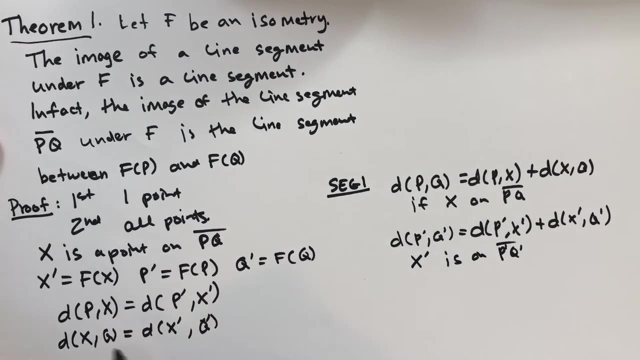 the distance from p prime to x prime plus the distance from x prime to q prime. okay, So that implies that x prime is on p prime, q prime segment. okay, so this shows that if we take a single point, x, so we say x is a single point. 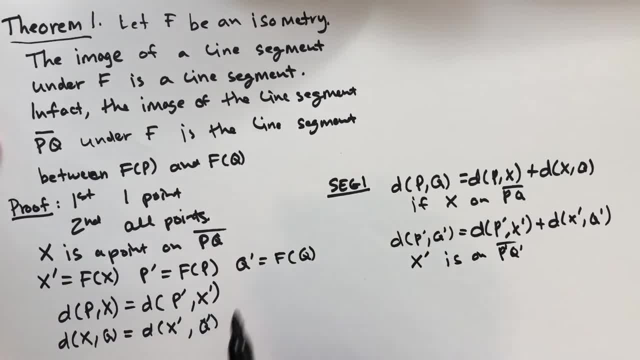 then, because distance is preserved, did i write down- i think i missed one here. also, the distance from p and q is equal to the distance of p prime and q prime, right, so all those distances are the same because it's an isometry, and so we use seg, one that said this, and so we were able to translate. 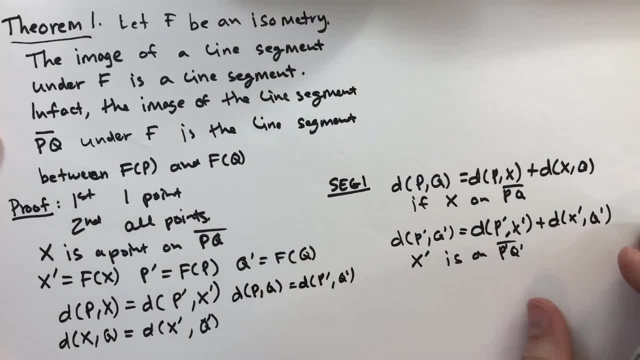 it. that to that. so x prime is also on p prime, q prime. but this isn't enough. we need to prove this for every single point. okay now, to prove that every single point on this line segment p prime, q prime can be expressed as an image under the f is okay. um, so if we take x prime to be a point, 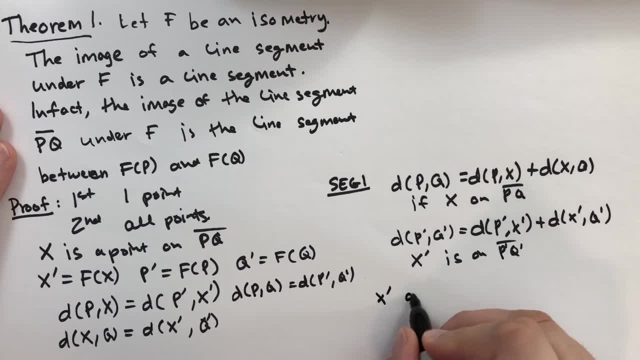 on p prime q prime at a distance r. so we take x prime is on p prime, q prime at distance r from p p prime. i mean okay. then that question is what is the distance from p to q prime at a distance r? corresponds with the point x on p q at the same distance r. 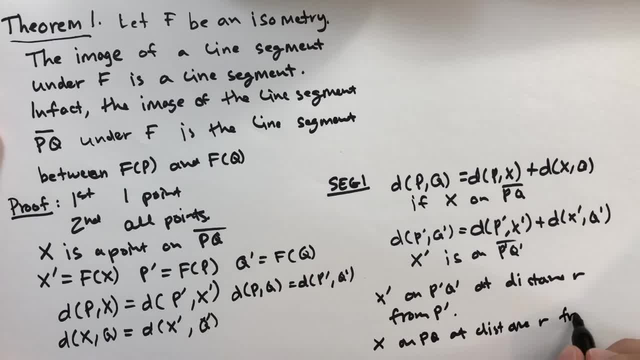 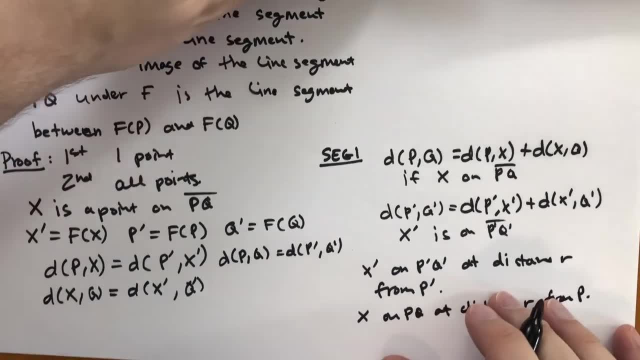 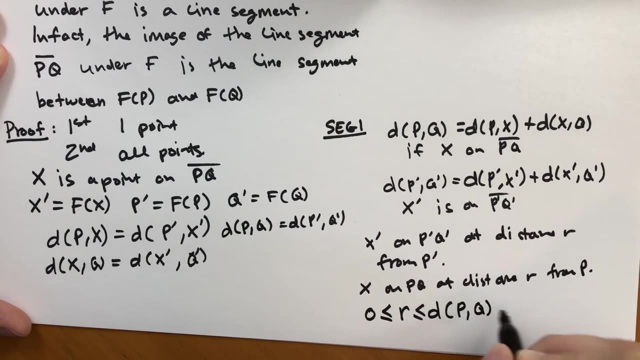 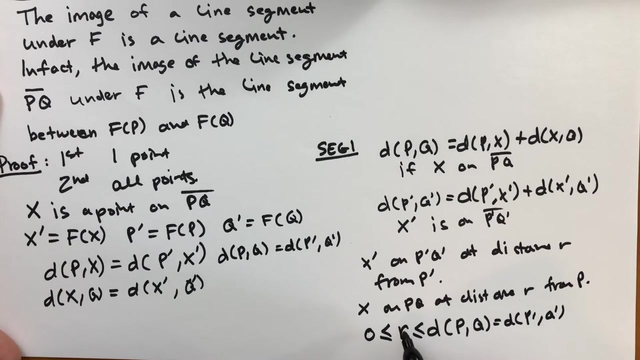 from p. okay, and so since r- there's not a lot of room here- push this up a little bit. since zero must be less than or equal to r, less than equal to the distance between p and q, which is equal to the distance from p prime to q prime, then this proves that for every value of r, every real number, 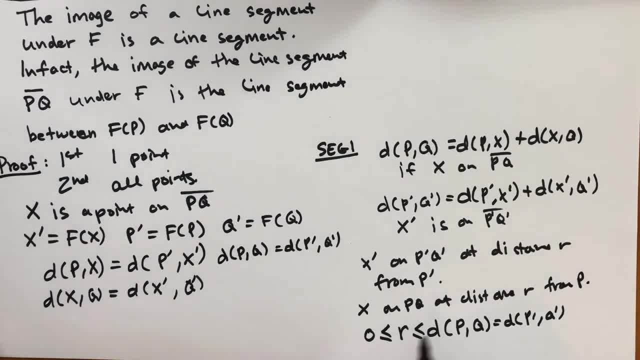 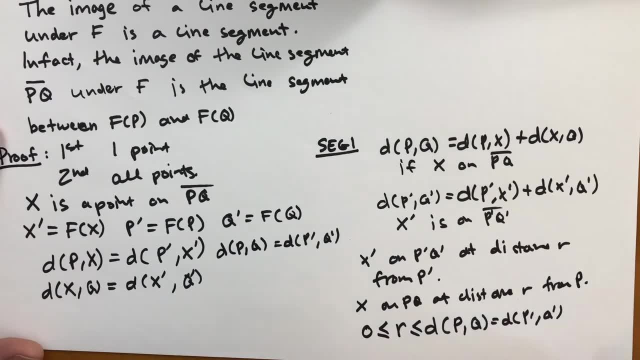 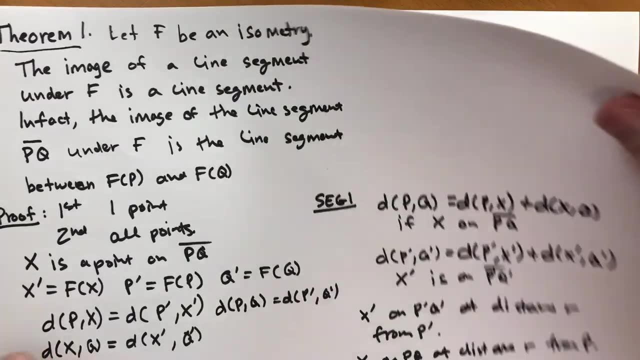 that you can use for r between this range. then there is a point that corresponds with the point on p prime, q prime and vice versa. so that is a proof that will cover every single point. all right now there's a remark here already at 15 minutes, but i debated making this video into. 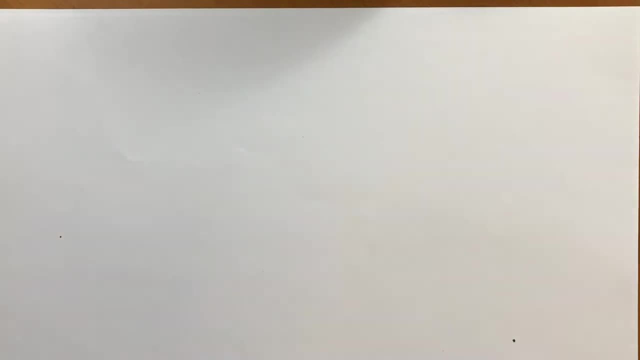 segments, but i think i'm just going to go make a long video. so all right, remark. he makes a remark here. he says: in this proof we want to show that two sets of points are equal and we have followed a standard pattern, namely we have proved that each 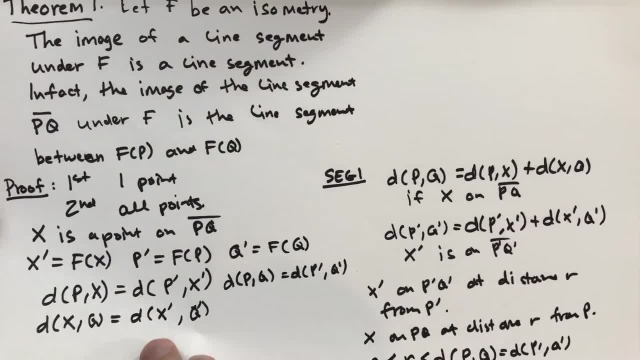 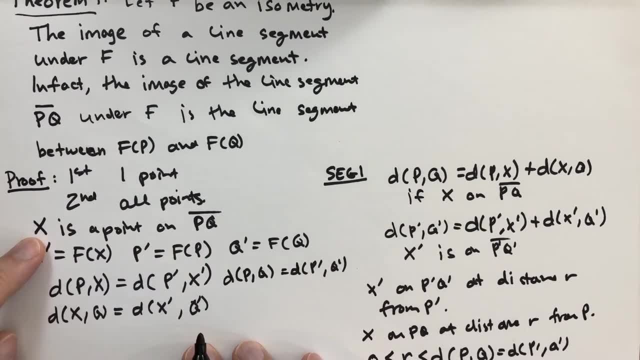 one is part of the other and this pattern will be repeated other so this pattern where we first prove it for a single point and then prove it for all points, where we take just any point in that segment or in that group of points and then we extend the the proof out for all possible points. 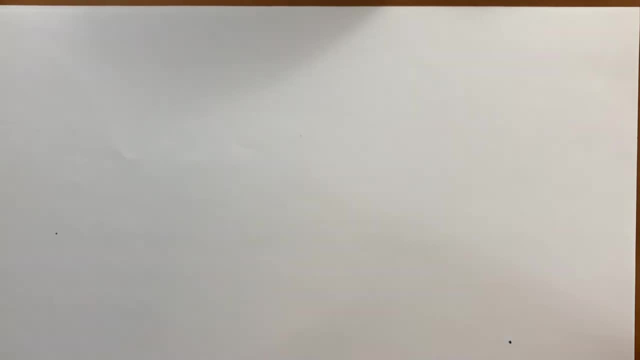 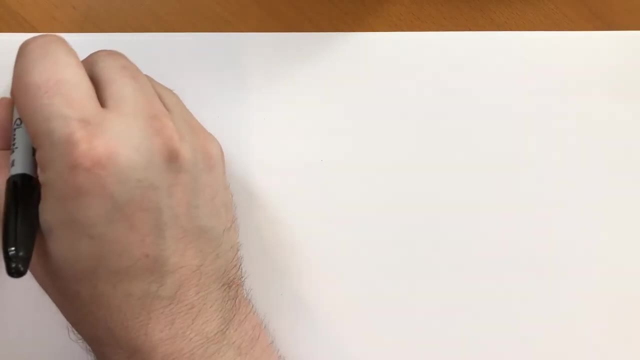 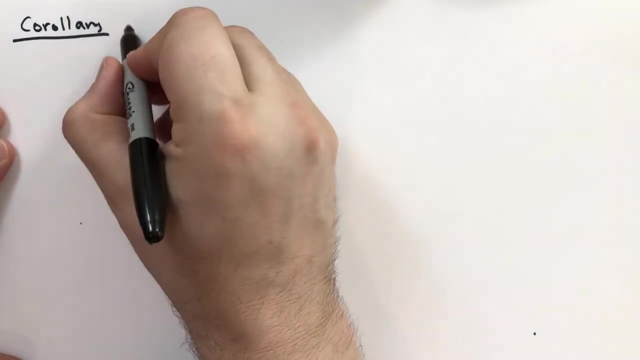 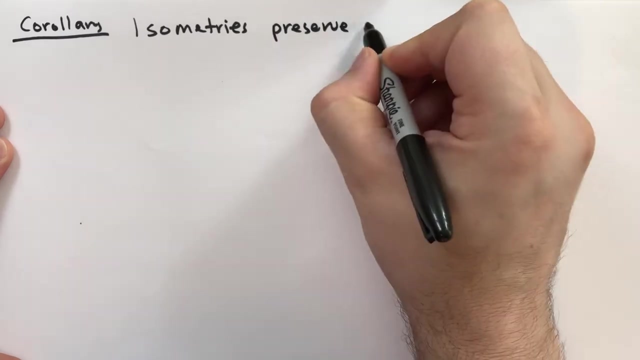 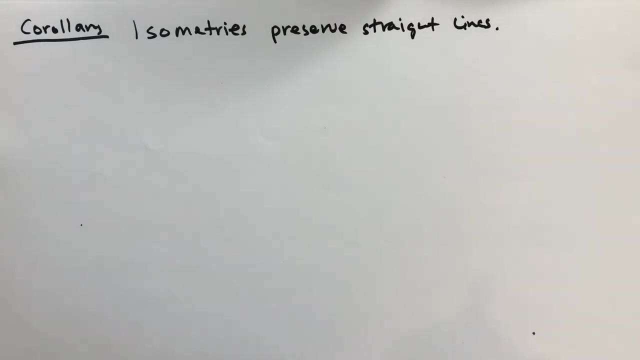 right then, that's the pattern that you generally follow with these kinds of proofs, so it's a nice little pattern to use. uh, corollary, and isometry preserves straight lines. so this is an interesting corollary. okay, isometries preserve straight lines, okay. in other words, if l is a straight line in the plane and f is an isometry, then f of l, the 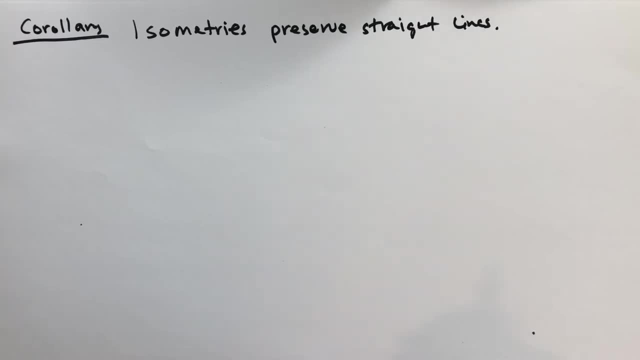 image of l under f is also a straight line. if l is the line passing through two distinct points, p and q, then f of l is the line passing through two distinct points, p and q, then f of l is the is a line passing through f of p and f of q, and we'll leave that proof to you as an exercise which. 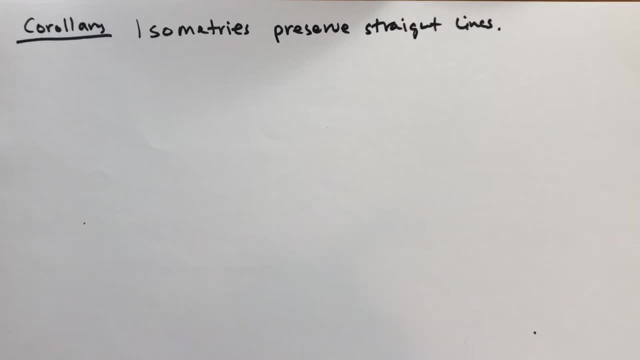 should not be difficult to prove. so I encourage you to either pause the video or, after this video, to go back and try to prove this for yourself. I think it is one of the problems. I don't know that it is one of the problems, but I think it is. let me review really quick. 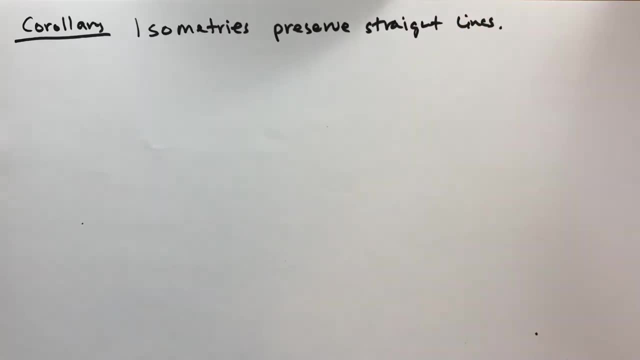 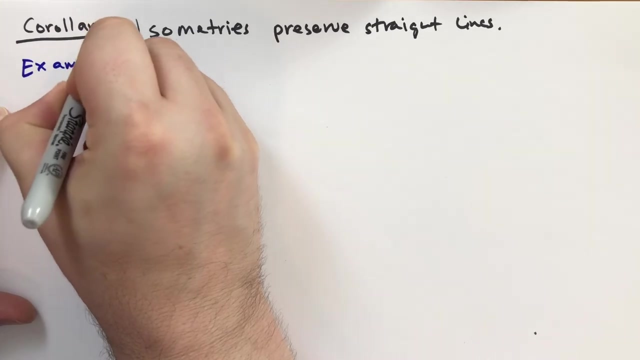 uh, no, it's not. it's not one of the problems, but there is an interesting problem that I want to get to. okay, try not to make this video too long, please. that's what I want to do. next, an example. there's a cool example here. example has a p in it. let o be the point of an intersection. 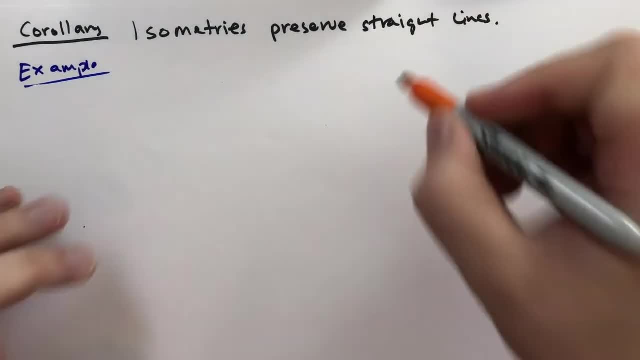 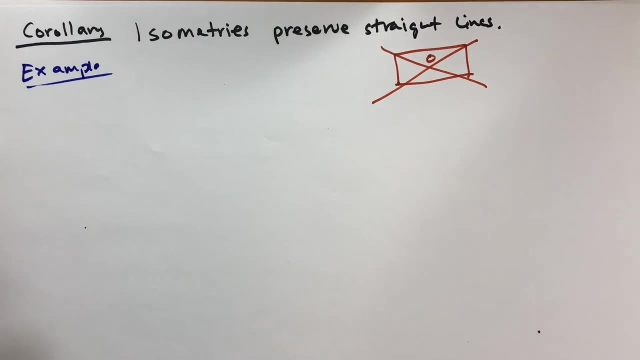 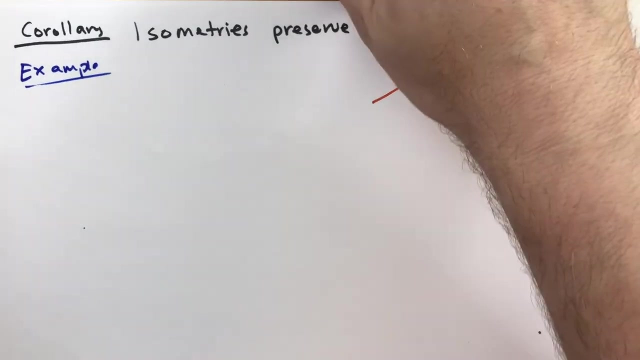 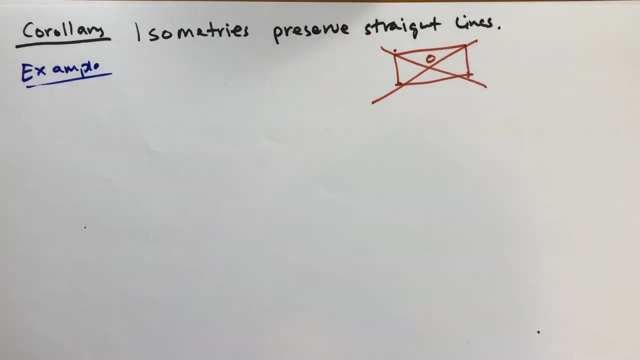 of the diagonals of a rectangle. so let's draw a rectangle, we have diagonals and o is that point where the two diagonals intersect. okay, if we reflect uh through o, then the opposite corners are mapped on each other. so this corner goes over here and this corner goes over here, and vice versa. okay, and because these two line segments 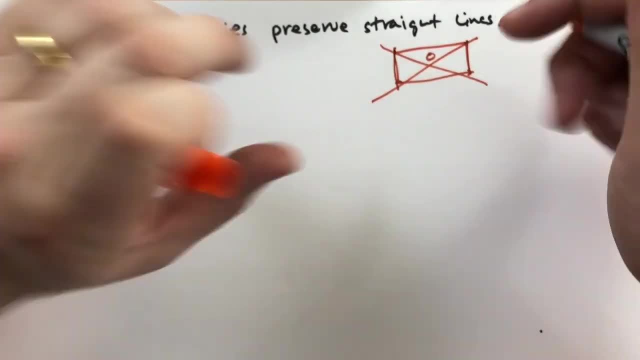 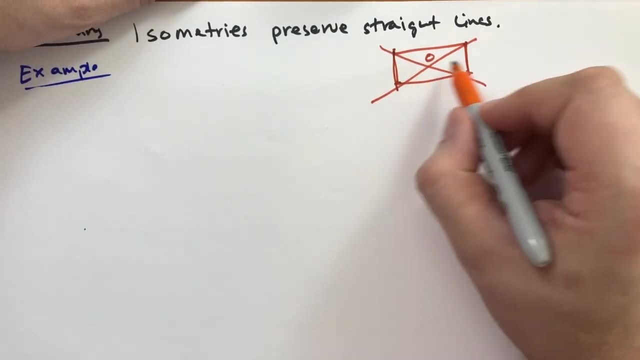 have points that map to each other. even though the line segments have to flip, they're the same line segments on the opposite side. so this reflection through the point is that and this reflection through the line, through the point, is this and same thing for the top and the bottom. 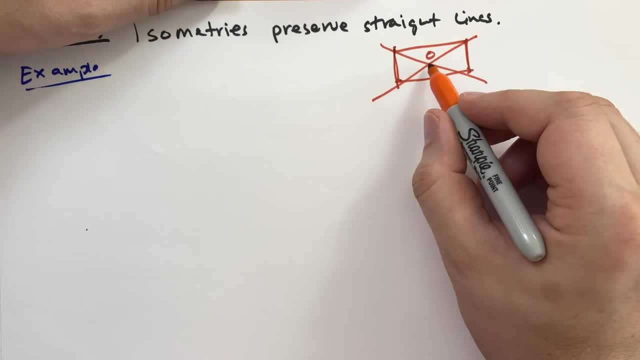 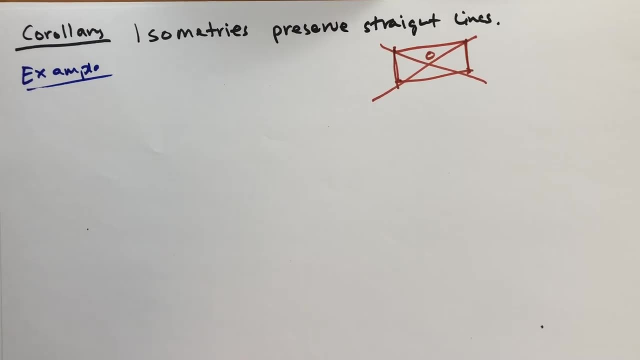 and therefore, even though reflection through through a point only has- uh, what are they called fixed point o, it's the only fixed point. this shape, the rectangle that centered on o, is also like a fixed shape. it's a fixed set of points. even though each point doesn't map to itself, you end up with the shape. 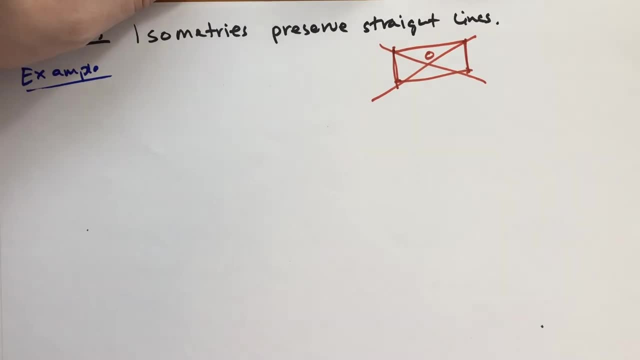 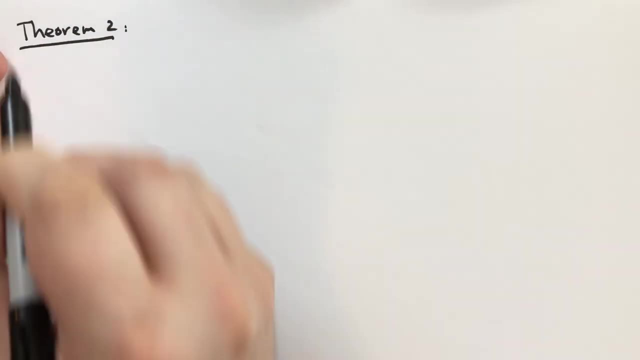 that's the same as what you began with, so that's a pretty cool example of interesting things. theorem two: theorem two states that if f is an isometric attacking frequency and then f is a Lorentz z important GNR order restoration, a reference zero, no case. 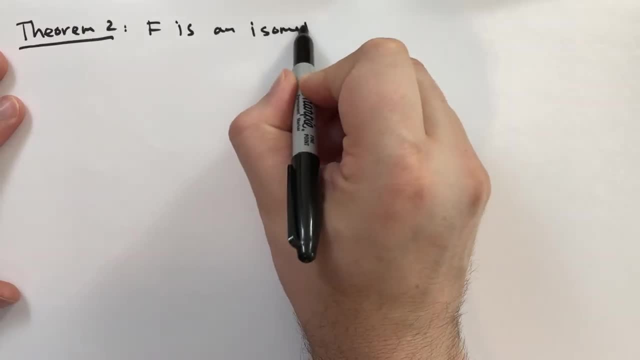 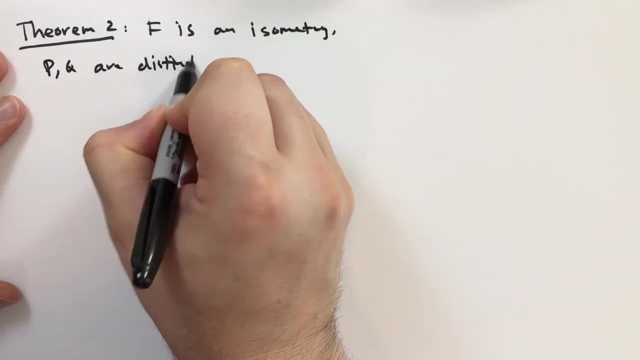 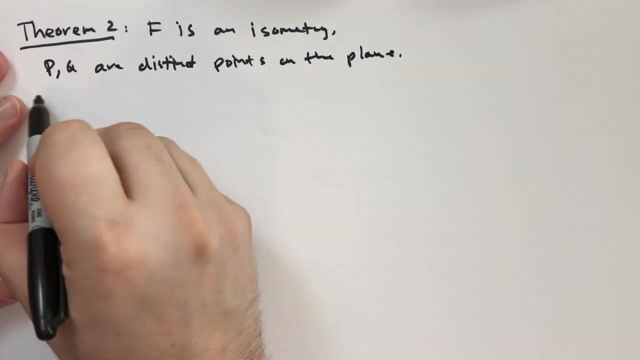 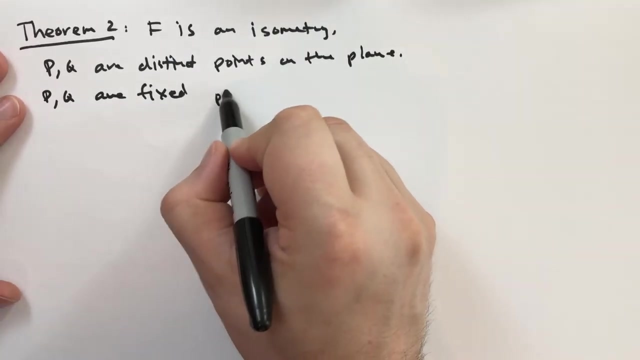 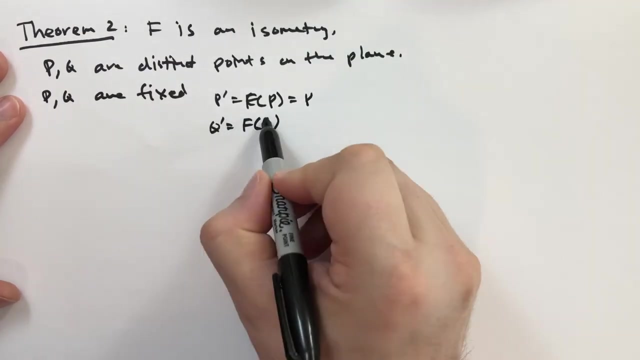 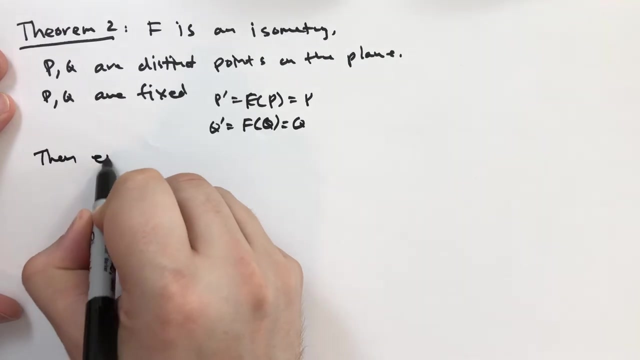 and P and Q are distinct points on the plane and P and Q are fixed points. okay, that means that P prime, which is the mapping of F through P, is equal to P and Q prime, which is the mapping of F on Q, is equal to Q. so those points don't change. when you map them, then every point on the line passing. 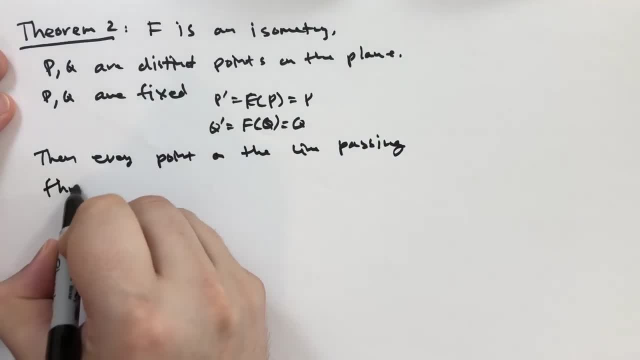 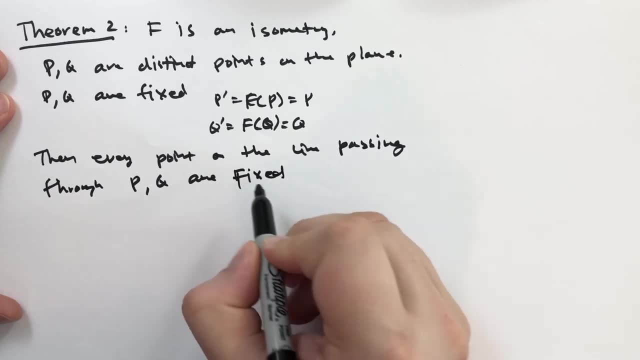 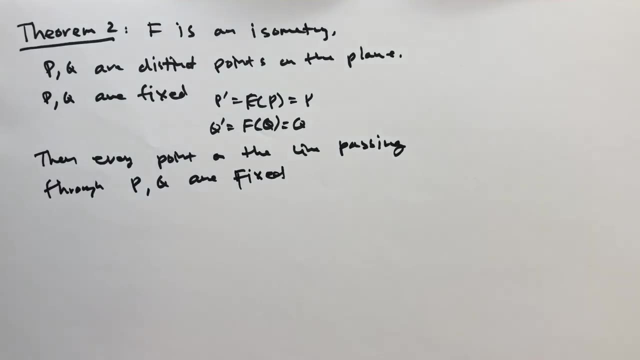 through, P and Q are fixed okay, so they also have that same property. in order to prove this, we're gonna take a look at a picture here. so suppose we had a line we use orange, we had a line and that's P and that's Q. so we're gonna consider three different cases, okay. case one is the line. the point lies between: 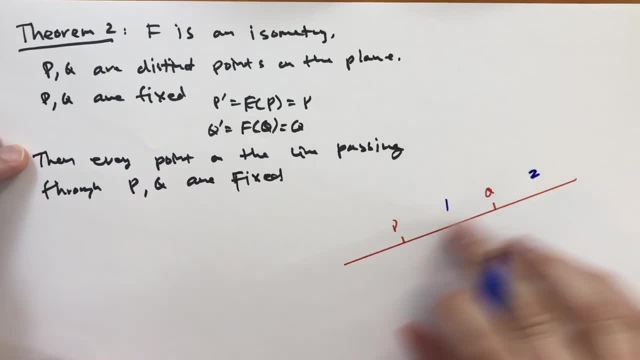 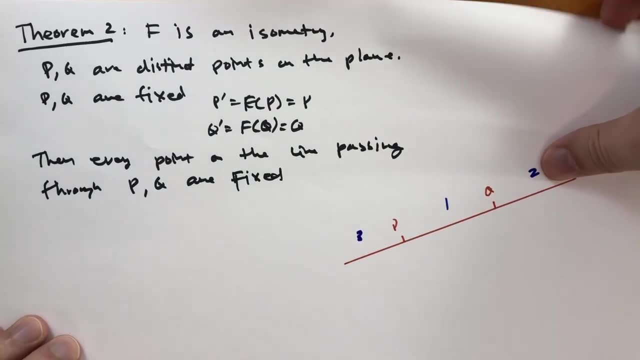 these two points. the case two is the line sits beyond Q and the point between these two points sits beyond Q, and case three is the point sits beyond P. okay, so we're going to consider those three cases. all right, let's go through these rather quickly. they're not too difficult to. 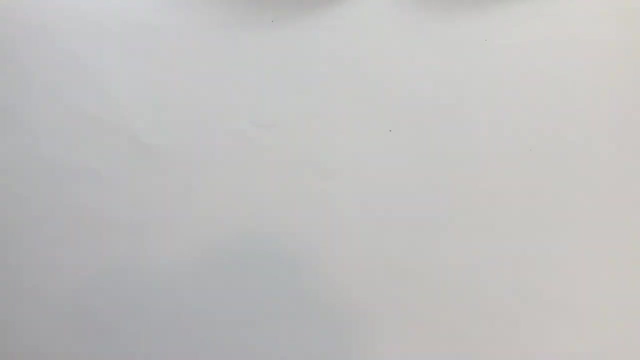 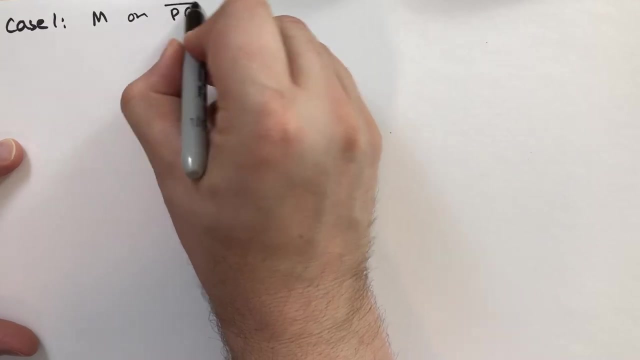 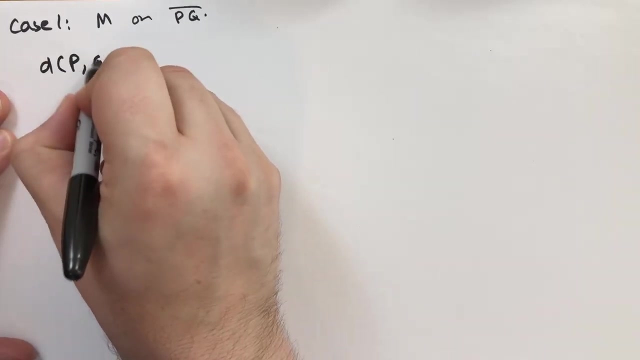 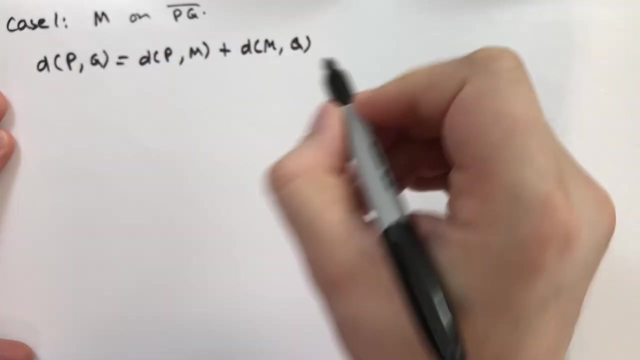 understand once we understand what we're doing here. so the first case, so case one. so M is on PQ, the line segment PQ. okay, so we note that the distance from P to Q is equal to the distance from P to M, adding the distance M, Q, and this is from seg one. that's from the seg one, proof that we did way back. 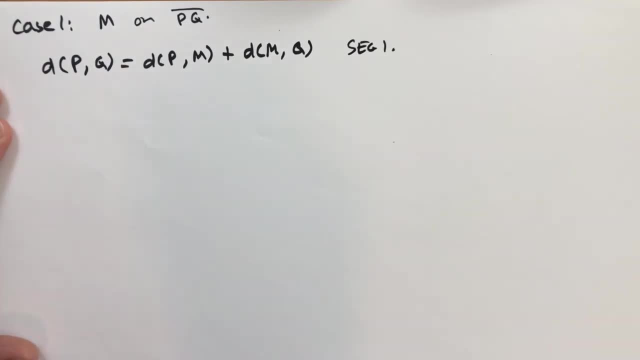 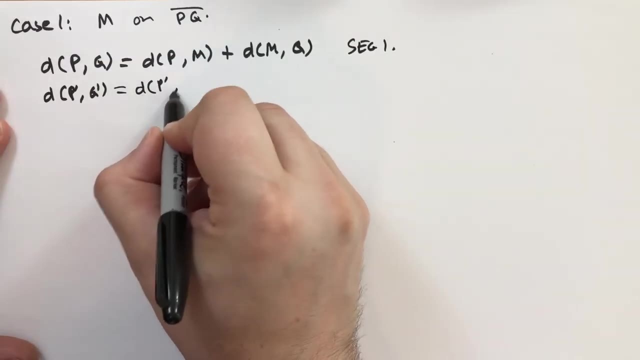 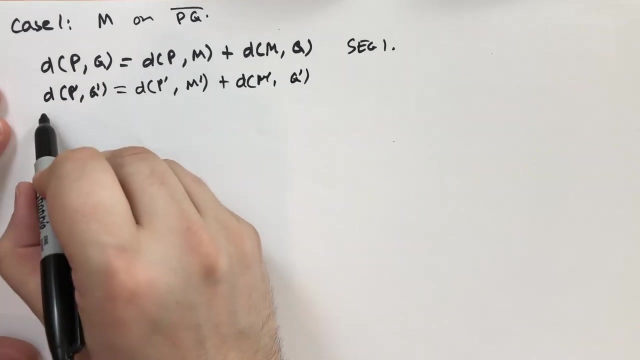 when in the last section, I believe, maybe the section before, I don't remember anyway. so the distance from P prime to Q prime, which are the same points, is equal to the distance P prime to M prime plus the distance from M prime to Q prime. okay, but we note that this is the same. so this is: 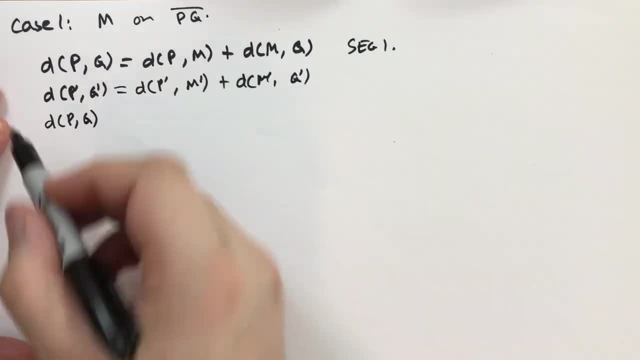 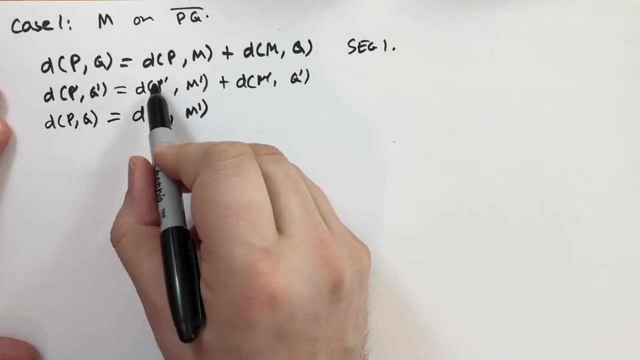 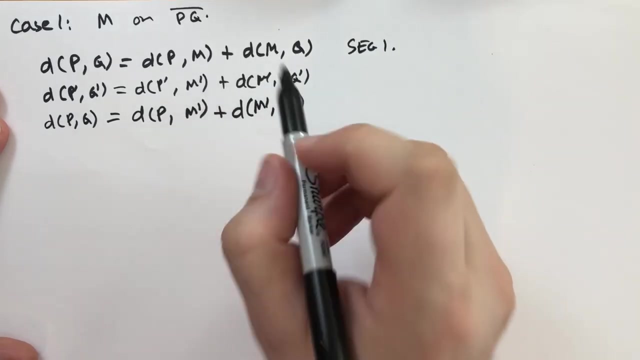 the distance from P to Q is the same as P prime, Q prime, because those are fixed points. it's an isometry as well. but more importantly, the distance from P to M prime is the same because P and P prime are the same points. and the distance from M prime to Q is the same because Q and Q prime are the same. 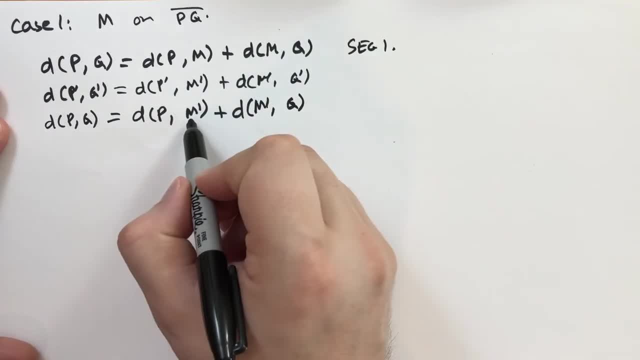 okay, so this has to equal that the distance between these two points is the same, and the point lies on the line. therefore, we must conclude that M prime is the same as M, why? well, let's draw a little triangle here. let's suppose that it weren't the case, right? so we have. 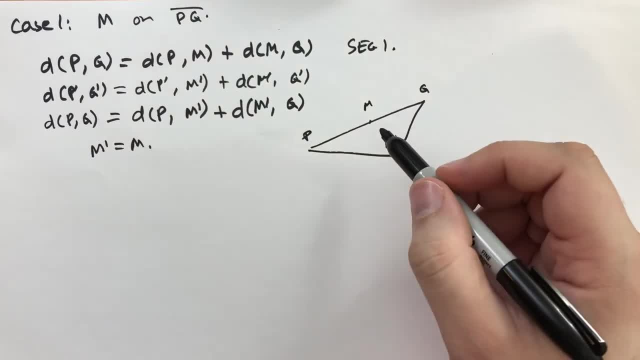 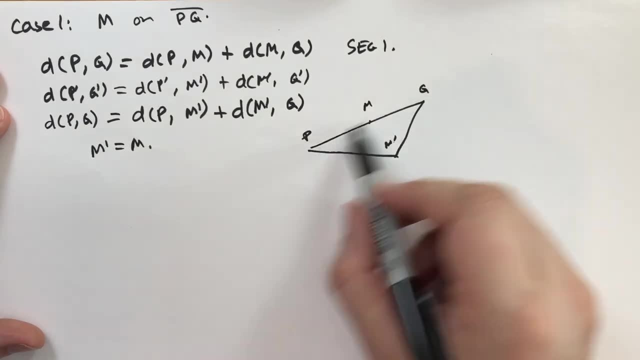 M over here in M prime. okay, so M prime and M are not the same points, they're not fixed. okay, so the distance from P to M prime and the distance from M to Q prime should be greater than the distance from P to Q. but it's not. it's the same. therefore, M must lie on them on the line segment. in fact it. 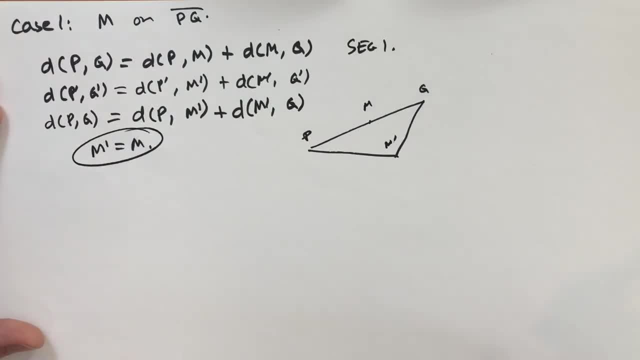 must be the same, okay, so those two points are the same. for case one, okay, case two: we say M is beyond Q on the line. okay, so in this case we have basically this: we have D, we have P, we have Q and we have M, and maybe M prime is out here somewhere, maybe it's a different point. so 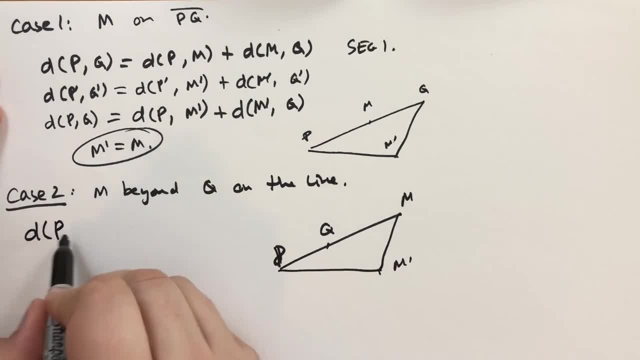 we're going to draw like that, okay, so we note that the distance from P to M is equal to the distance from P to Q plus the distance from Q to M. okay, and applying isometries, so we get P to M prime is equal to the distance between P and Q, because P and Q and P prime and Q P. 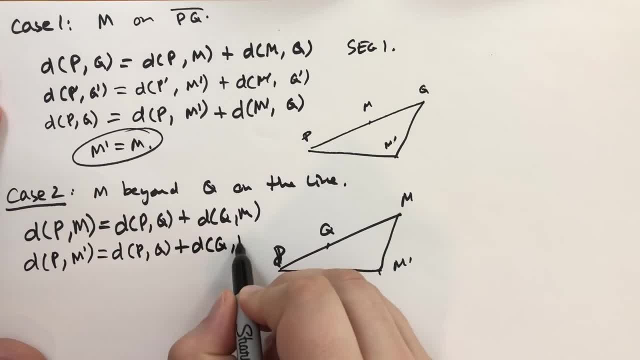 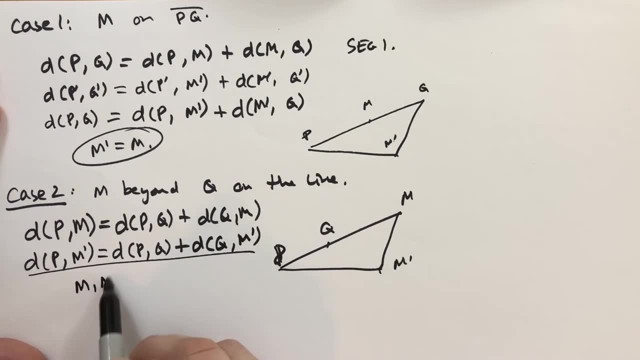 prime and P and Q, prime and Q are the same points and is the same as the distance from Q to M prime. okay, and because this is true, because these are isometries, then it must be true that M and M prime are the same. okay, so these two points are actually the same, because 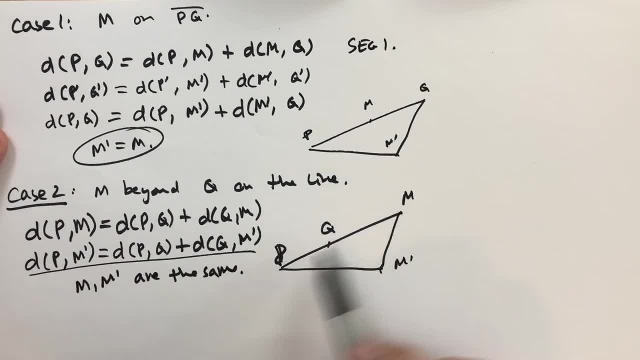 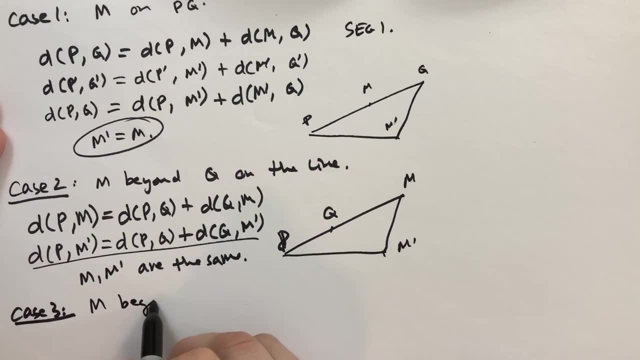 the distance is add up, it's not the triangle inequality. where this distance is greater than that, we just say m is beyond p on the line and we just follow the same proof before, except we substitute p and q with each other. so it looks like this: we have q, we have p, we have m, we have m prime. same, same deal. it just works out to be: 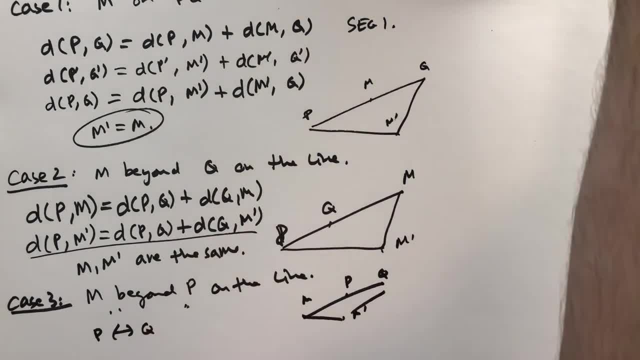 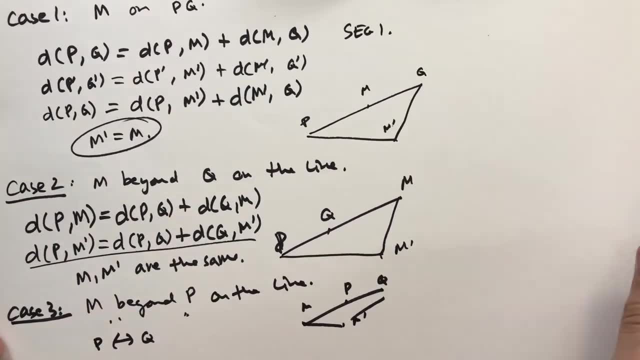 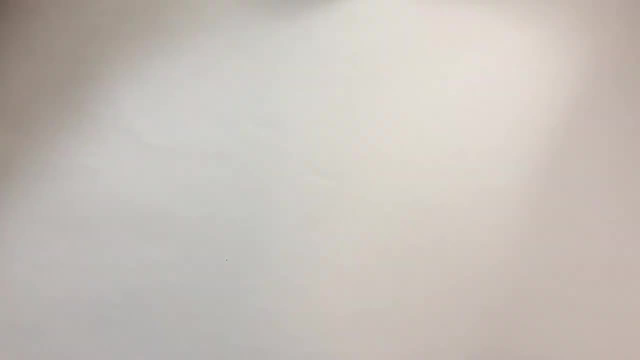 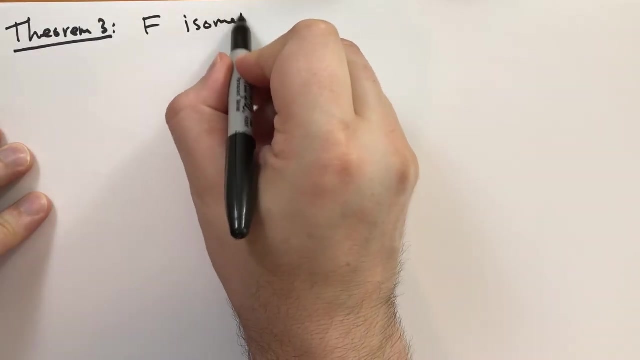 the same. okay, so that's a pretty simple proof to prove that um distinct points, fixed points. if you have two fixed points at every point along the line is also a fixed point. pretty cool, all right. theorem three theorem, three states: f is an isometry, p, q and m be three distinct points. p, q, m are distinct. 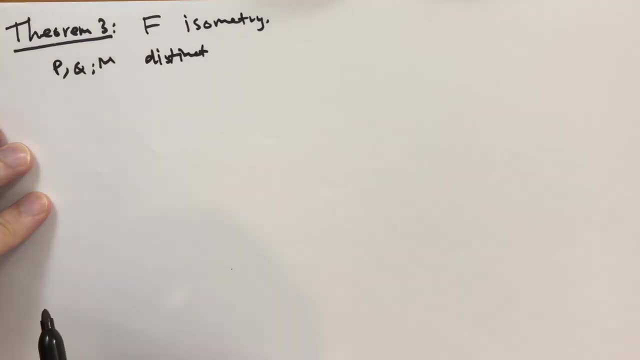 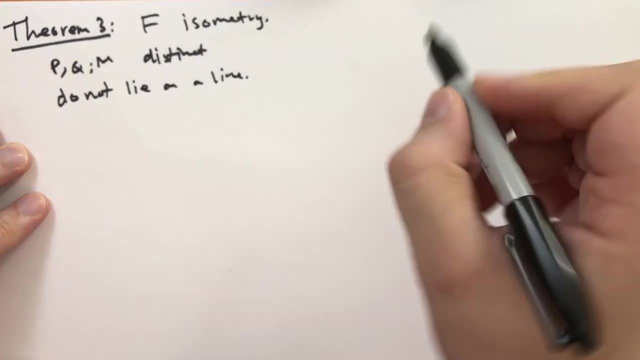 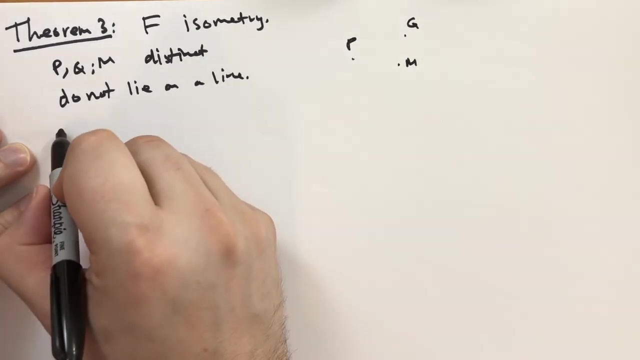 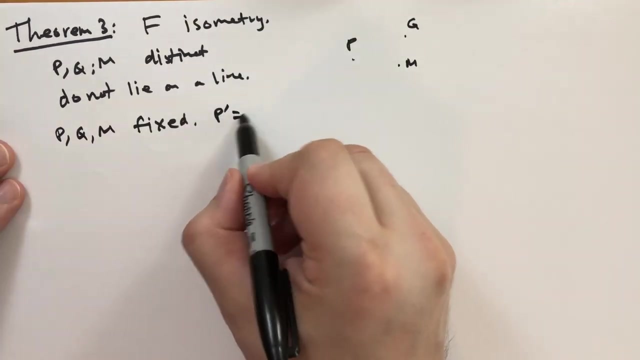 and they do not line a line. this is popularly known as a triangle. okay, and assume that p, q and m are fixed. okay, so that just says that p prime is equal to the mapping of p through f, which is the same as that and the same for a. 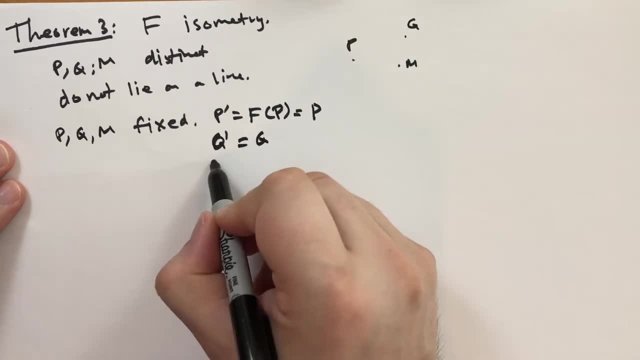 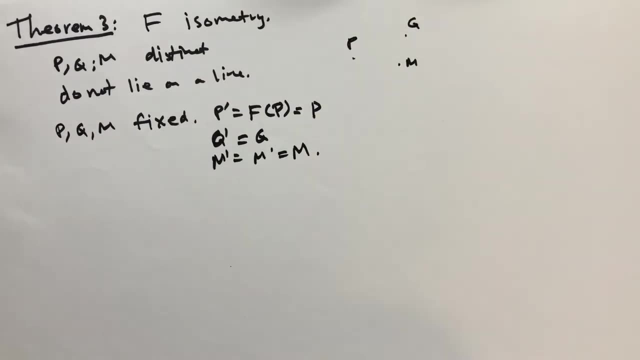 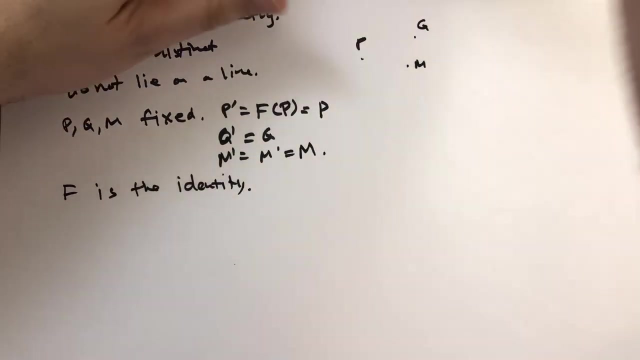 q prime is equal to q and m prime is equal to m, m, not m prime. okay, so the theorem says that f is the identity mapping. basically every point maps to itself. every point is fixed. therefore, f is the identity, the proof of this. so we draw two lines. 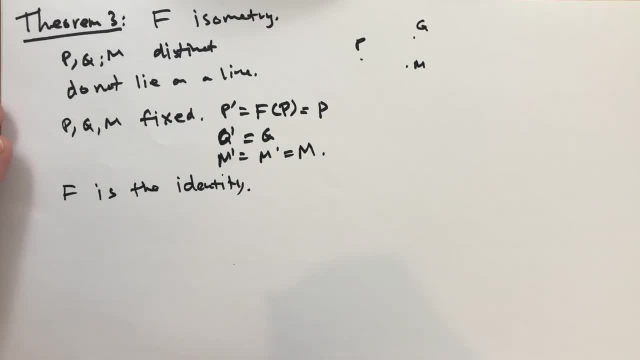 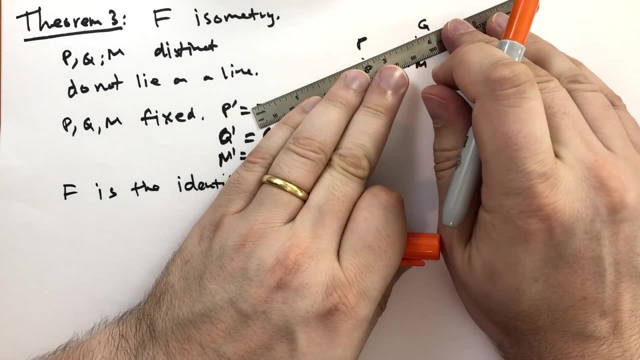 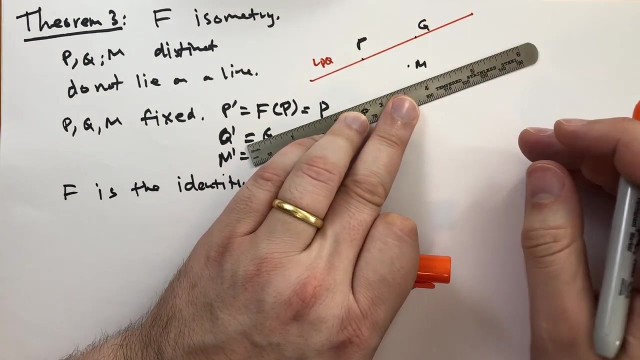 l p q and l q m. so let's draw l p q. we use a different color. let's not use black. it'll make this messy. let's use a nice orange here. l p q- this is l p q and we're going to have l q m. 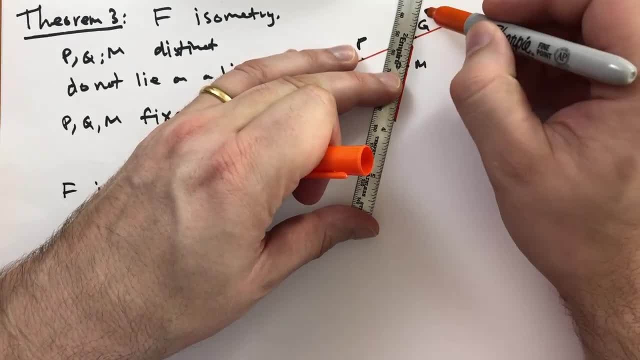 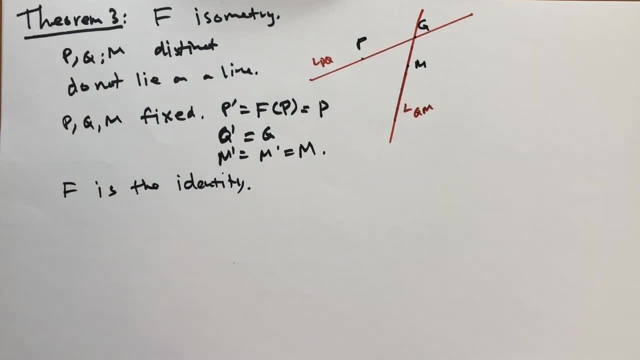 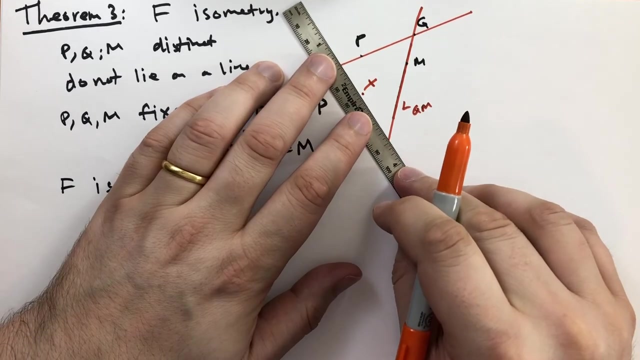 all right, so we have those two lines. x is a point. we're going to choose x such that it doesn't lie on either of these lines. let's choose x out here, okay, and we're going to draw a line that passes through these two. it doesn't matter what line, we choose any line. 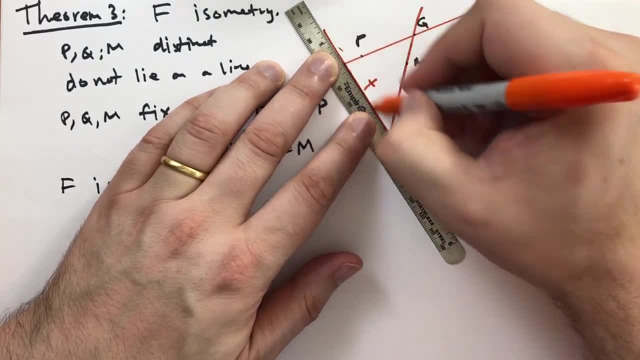 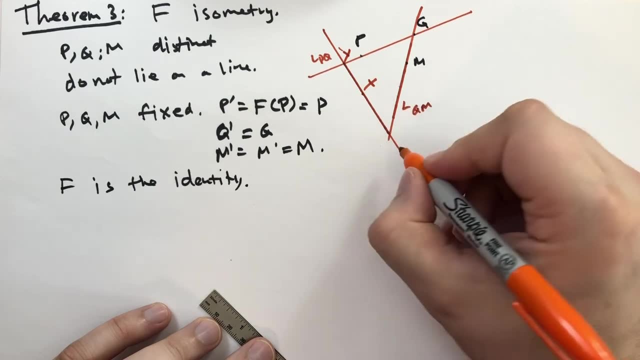 okay, passes through these two lines and through x. we're going to call one of these points, y. y is the one that's going to be the line that passes through the PQ. we're going to call the other, z, which is on QM. okay, so we have those points. 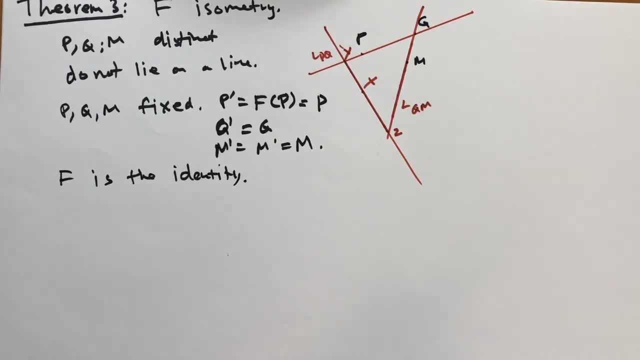 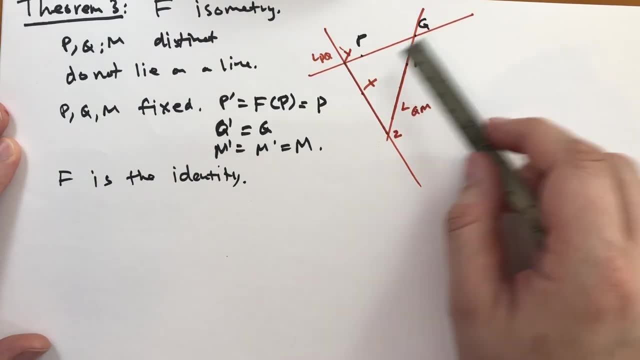 okay, by theorem two, every point on this line is a fixed point. in every point on this line is a fixed line. that's because P and Q are fixed points and Q and M are fixed points. so every point on these two lines are fixed points. so the Y is a fixed. 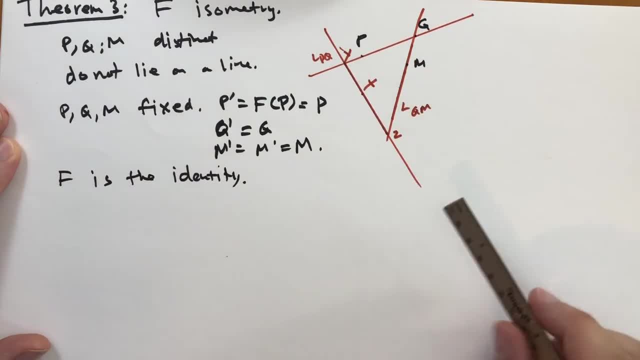 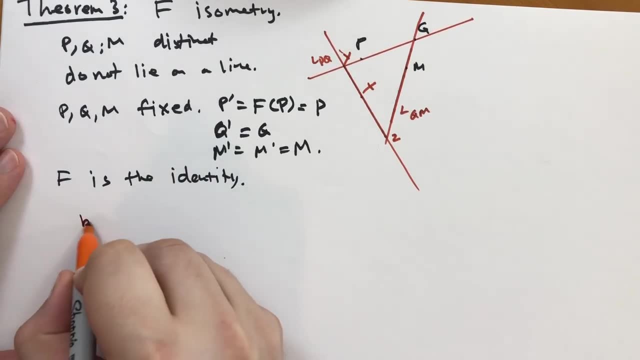 point and z is a fixed point. there for every point between the two lines, y and Z are also fixed points. therefore x is a fixed point. Okay, so because theorem 2 says L, P, Q, all fixed, that leads to Y is fixed. 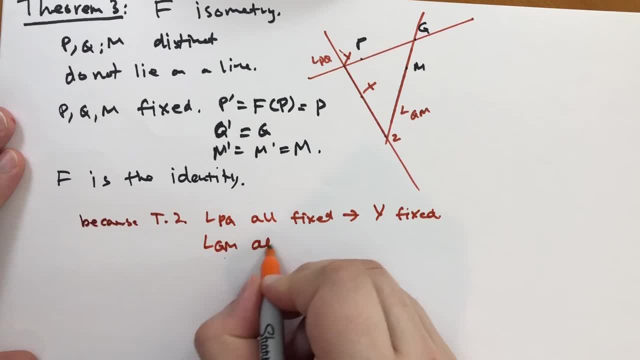 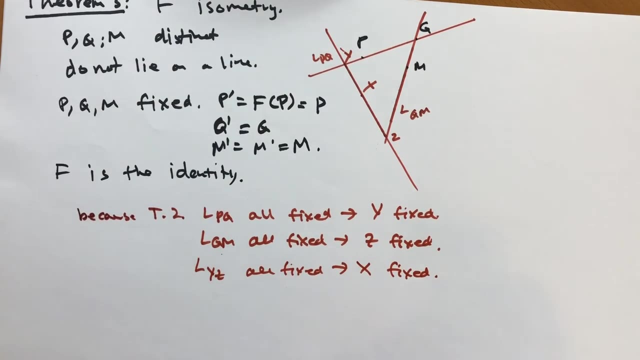 Because Y is on L, P, Q, L, Q, M are all fixed. Therefore Z is fixed. Therefore L, Y, Z are all fixed And that means X is fixed. Okay, that's theorem 2, right there. 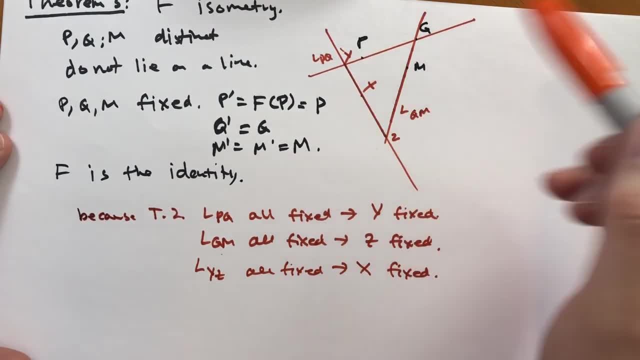 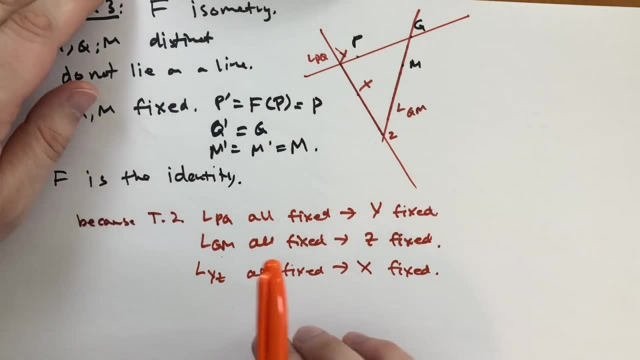 And so there's your proof that every point you pick, it doesn't matter where the line is, where the point is, what line it's on, it doesn't matter. You'll always be able to find a line that intersects between those two points and that point. 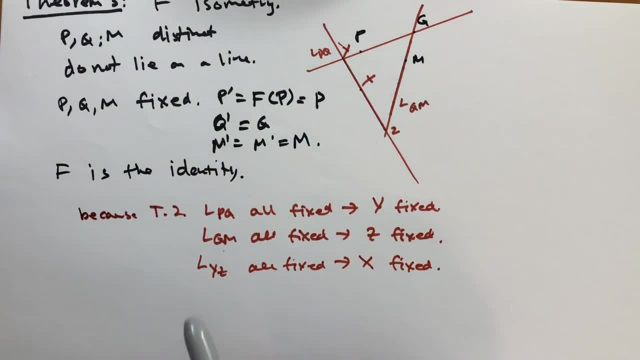 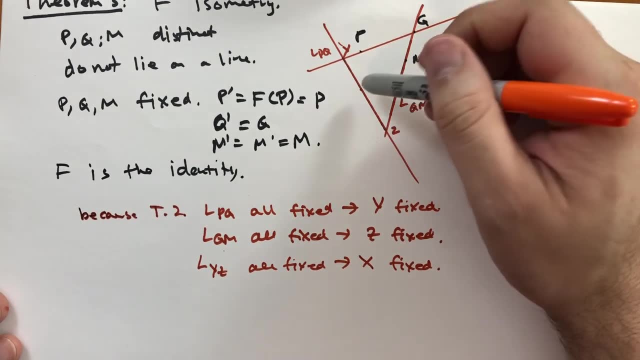 Well, that would be another proof altogether. No, it should be relatively obvious. You can always find: if you choose any point on L- P Q, you'll find another point that also goes through Q- M, Unless X is on P Q, in which case it would already be fixed. 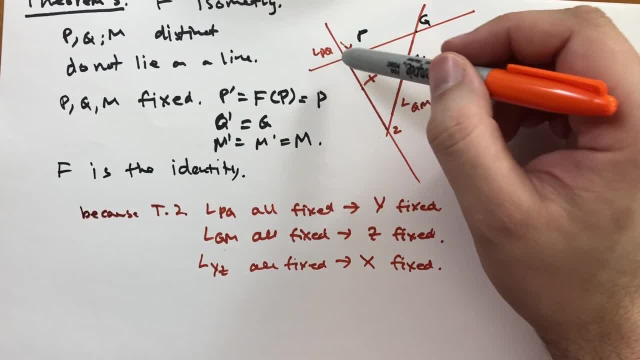 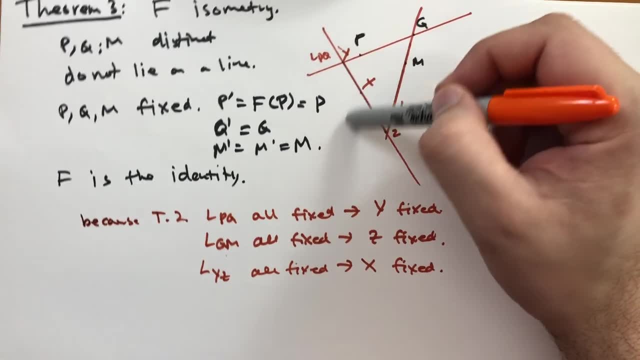 You wouldn't have to do that. So as long as X is not on these two lines, you'll always be able to find a line that intersects between those two points. You'll always be able to find a line that intersects both. Okay, there's one line, sure, that's parallel, but every other line is not parallel. 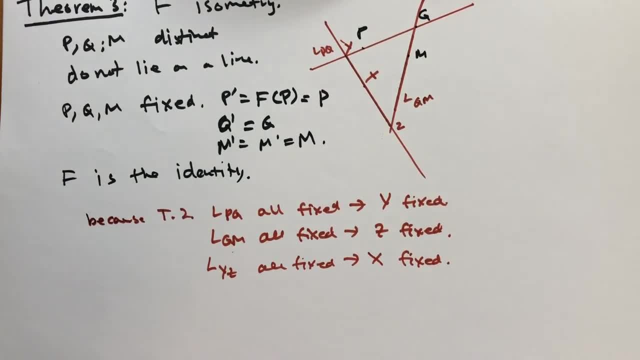 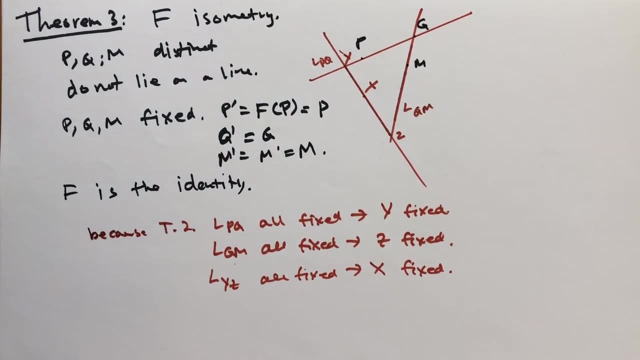 So that should work. Okay. remark: a very important core of this theorem will be stated when we have a notion of an inverse, of an astrometry, in section 4.. I'm going to talk a little bit about the exercises here. I want you to shift gears now with your education in math. 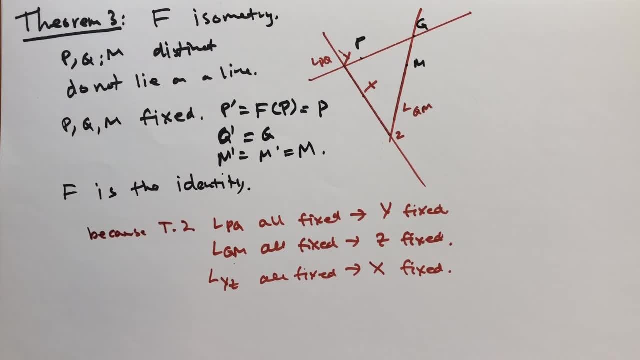 And I want you to stop thinking. I want you to stop thinking of solving problems and start thinking of proving proofs. okay, Really, every problem is a theorem to be proved. okay, The problem suggests to you: hey, here's a theorem. 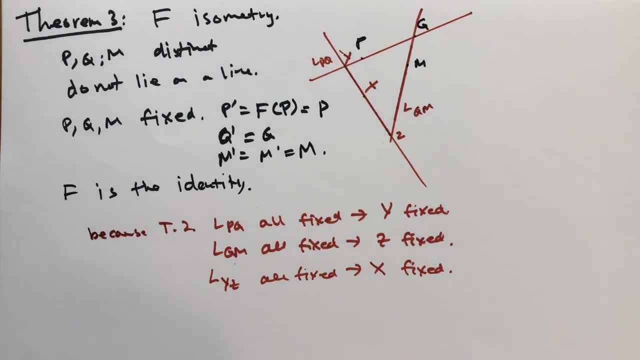 Would you please prove it? And too often I think we start off with our elementary and junior high school education and we get focused on finding the right answer, that we forget that really we should be using logic and we should be learning to use logical steps to find the right answer. 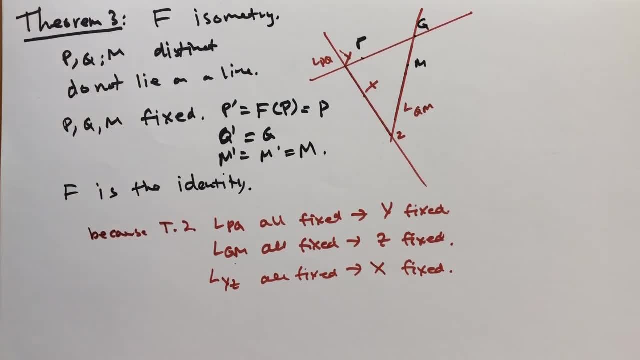 Okay, so these problems, these exercises are really great because these are almost pure logic. right, You have to apply logic to figure these out. So draw the image of a line segment under reflection through a point, through a line, and rotation by 90 degrees. 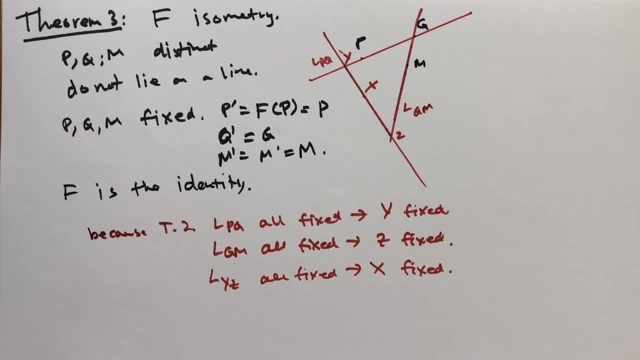 Pretty simple stuff. you know that should be pretty easy, And you can use the theorem that states that it doesn't matter what isometry you're using, the image of the line segment will itself be a line segment, And so you just need to rotate P and Q or project it, reflect it through a line or a point. 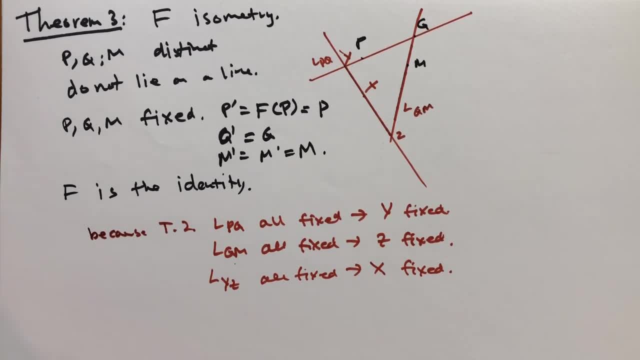 and then you'll be able to find your thing. Also, we do translation rotation by 80 degrees on the other side, on the other page. Okay, The next value of R is dilation by R in isometry. So there's one particular value of R for dilation, that is, in isometry. 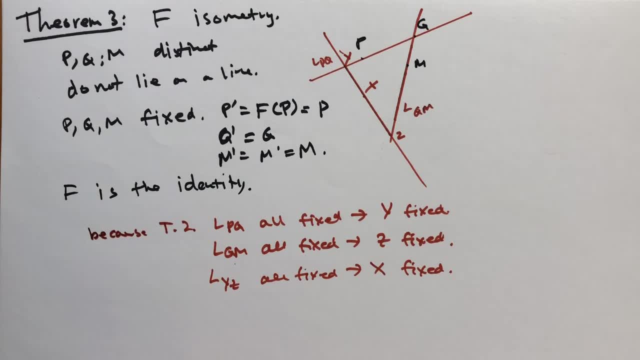 and you should be able to name the isometry that that is pretty easily. This one shouldn't take more than five seconds to figure out. Three: draw the image of a circle of radius R, center, P. Okay, And here we're doing circles. 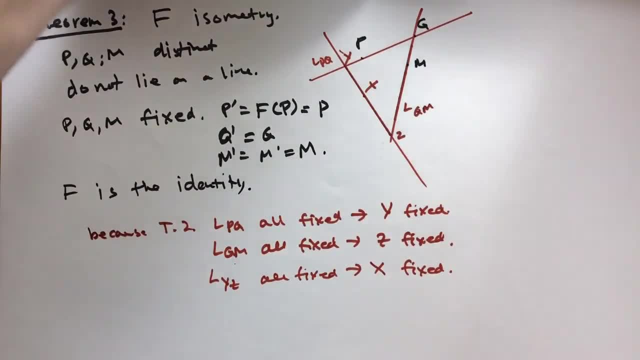 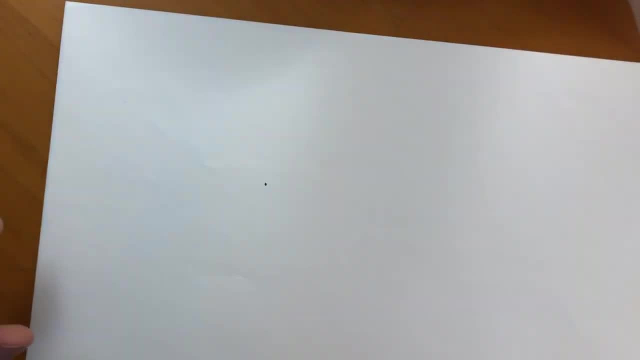 So, if you remember, with the circles, the circles are defined as the set of all points and they're a particular distance away from the center, right, And so when you have a circle, it says P and you have a circle that goes around at every. 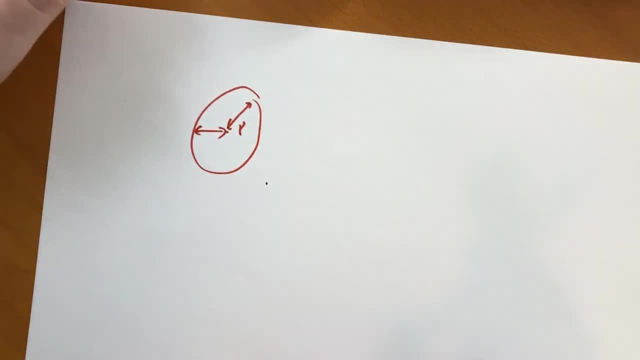 the distance from the center to every point is the same And since we're preserving, we're preserving distances, the circle won't get bigger or smaller. You just have to move the center point and that's your new circle, right? So we have a reflection through a center. 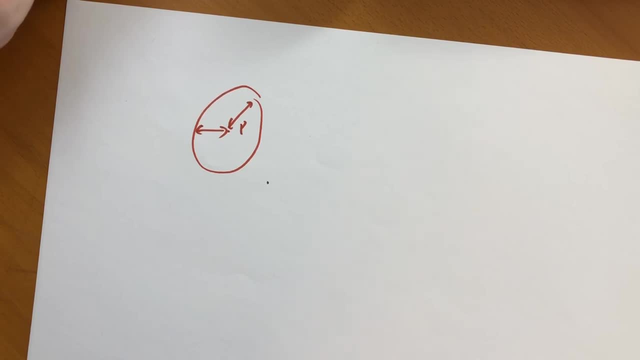 We have a reflection through its center reflection through a line reflection rotation, 90 degrees with respect to point O, outside of the circle, all these things. So that should be pretty easy and fun to do. It shouldn't take too long. 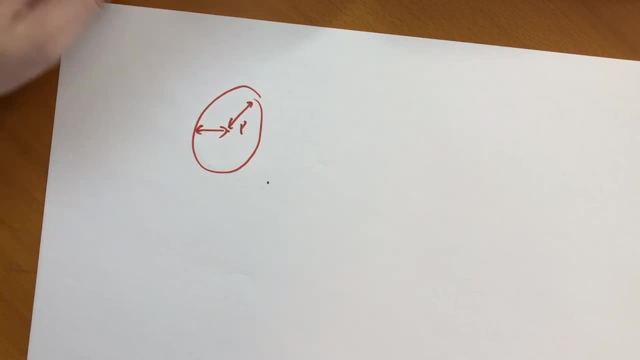 Number four: let L and K be two parallel lines. Let F be an isometry. So we have two parallel lines, L and K, Okay, And then we have an isometry, It doesn't say which one. All we have to do is prove that L and K are parallel. 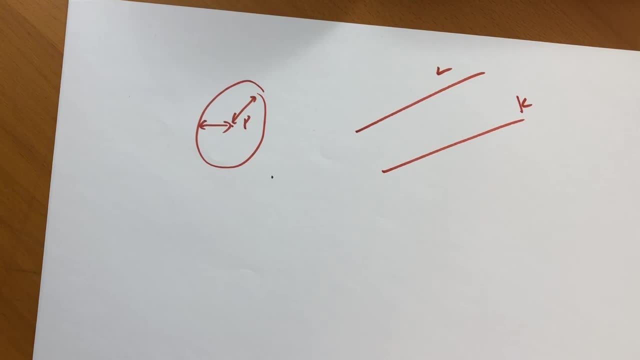 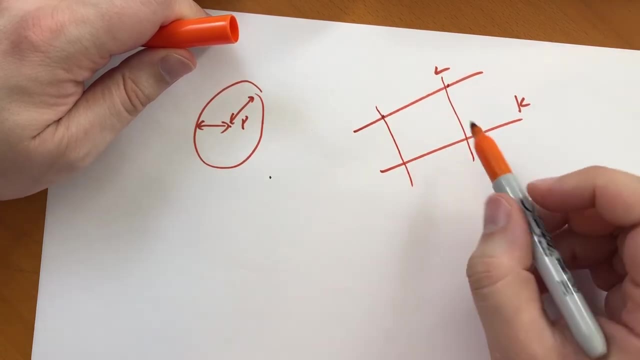 And how would you prove the two lines are parallel? Well, all you have to do is prove that the, if you draw perpendicular bisectors or not bisectors, if you draw perpendicular lines, right that these points are the same distance apart as these points. 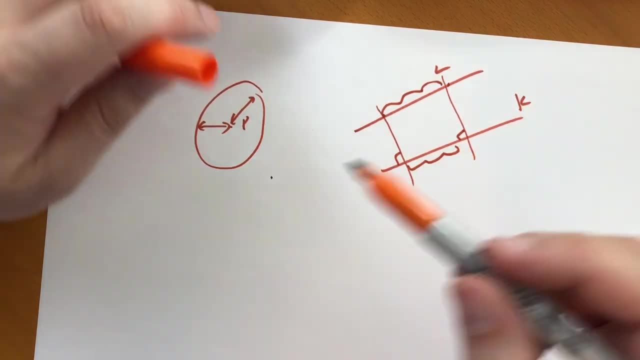 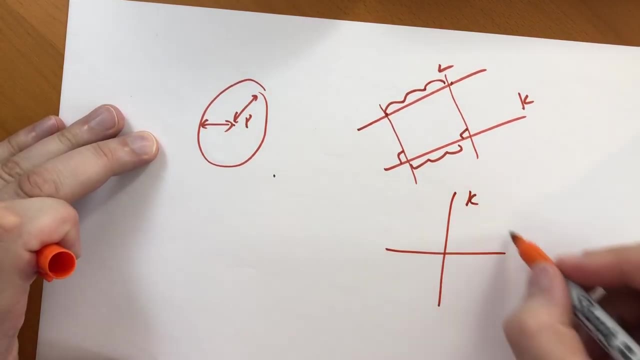 Okay, And you basically have a rectangle, And that's one way to prove it. You can probably think of some other ways. Okay, Five, let K and L be perpendicular lines. So number five you have: K and L are perpendicular, right. 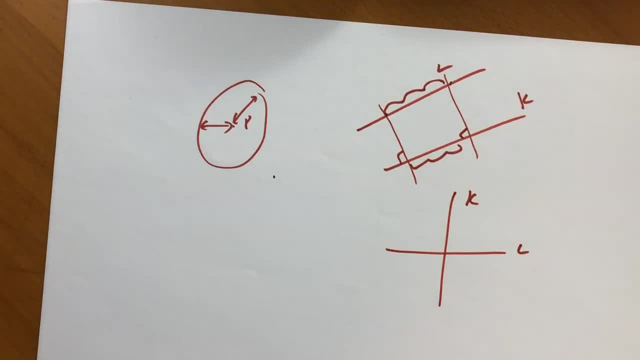 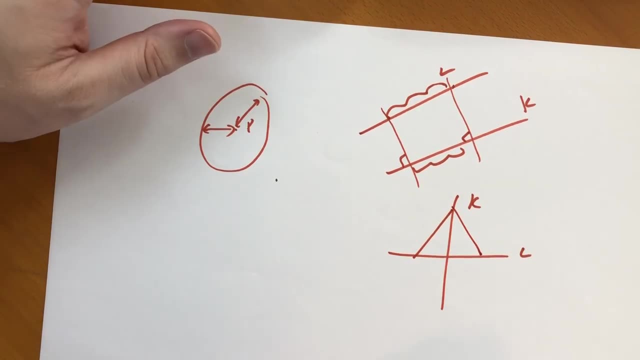 And let F be an isometry- Prove that F of K and F of L are also perpendicular. You might want to use the corollary of Pythagoras' theorem. Remember when we drew that shape like this? You might want to use that shape and use Pythagoras' theorem. 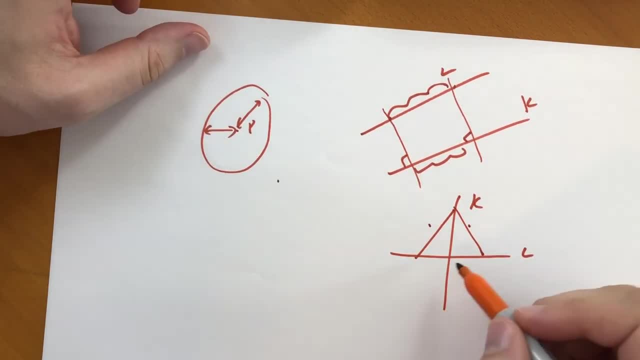 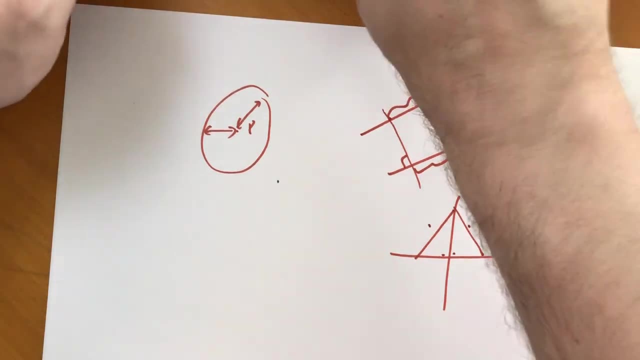 to prove that this distance and that distance don't change and therefore this is still the same angle. Okay, This number six. this is what I really wanted to get at, And this is a fun one. So the key of this problem is that last sentence there. 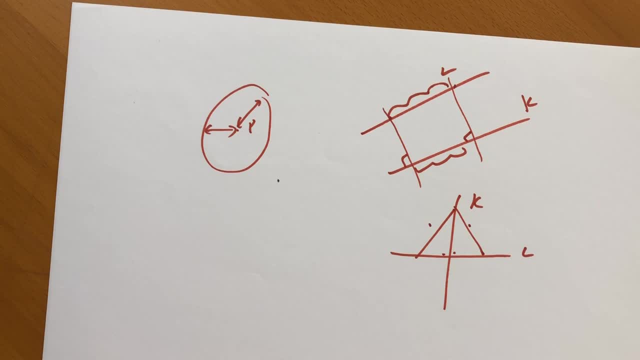 Aside from learning mathematical substance, you will also learn how to think more clearly and how to write mathematics in the process, Because he wants you to prove that you can define. you can define isometries in three space, the same way you can define isometries in the plane. 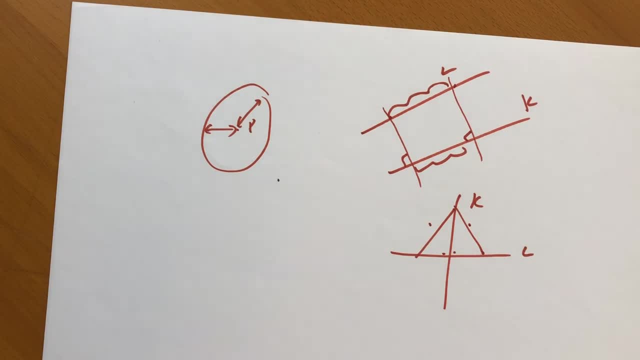 And you can also show that the theorems one and two that we proved work in three space. And he says: write this all up as if you were writing a book. So try to make this sound like you were writing a book, Make it look like the book. 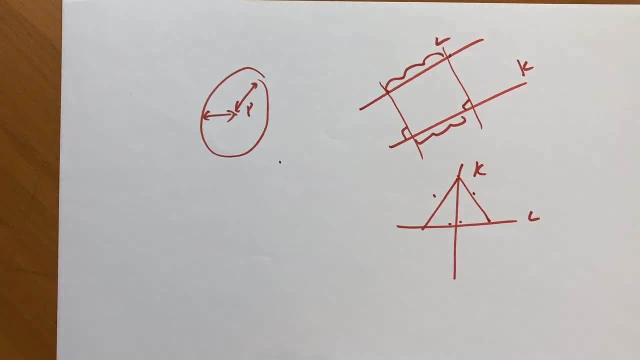 So number six: I encourage you to take a lot of time on number six and to try and make it sound like you actually know what you're talking about, that you're pretend to be for a moment that you're writing a textbook, And what would you write? 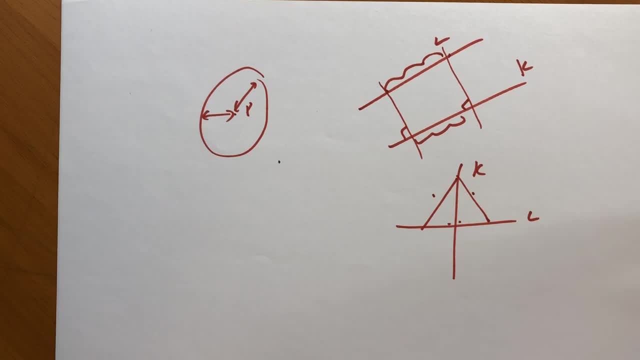 How would you put the statements together so that it makes logical sense? That's what I want you to think about. on number six, And the reason why I say pretend to be a mathematician is because by this point you should start to feel like a mathematician. 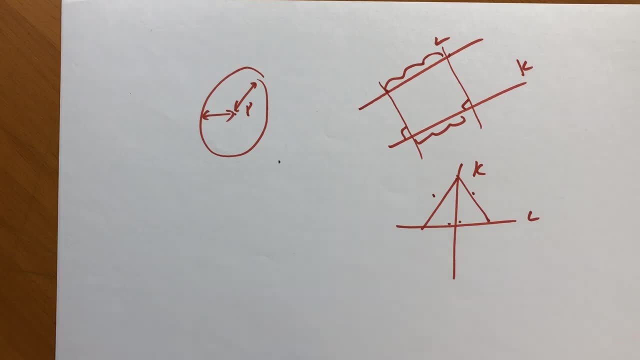 You should start to feel like you're more interested in proofs and not in just solving problems. Anyway, with that I'll let you go. Have a great day, Take care and bye-bye. Hey guys, thanks for watching this video. 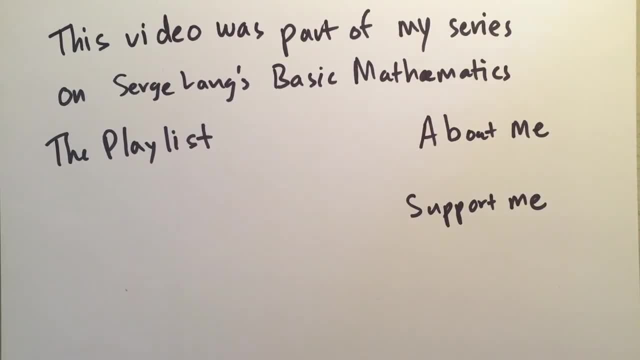 This video is part of my series of Sergey Lang's Basic Mathematics. You can click here to watch the rest of the videos in the playlist. You can click here to learn more about me And you can click here to support my channel. Thank you so much. Bye-bye. 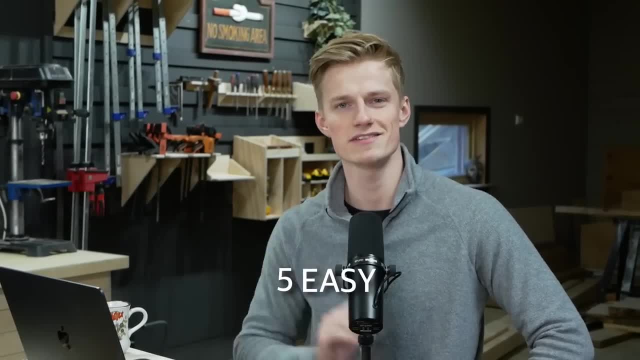 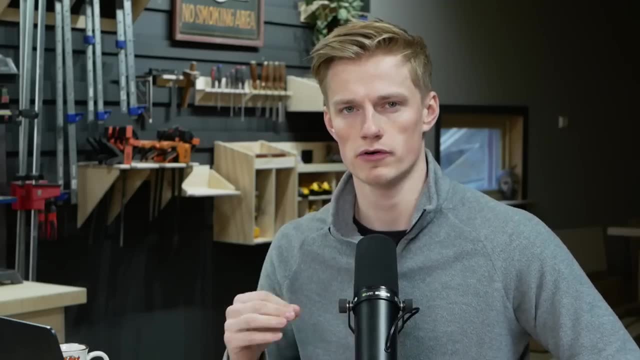 In this video I want to show you five easy woodworking projects that are selling really well right now. Some of them are projects that I'm selling myself and some of them are from sellers who are doing really well on Etsy. All of these will be pretty simple. They have a fairly 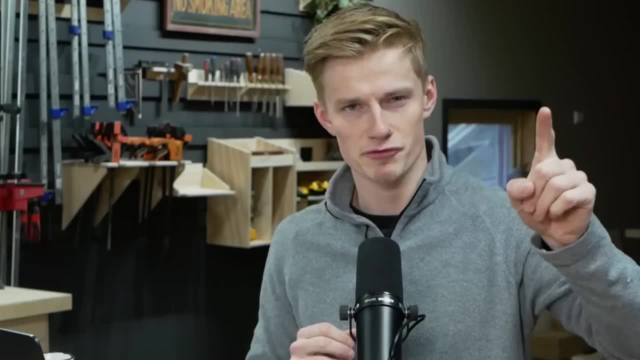 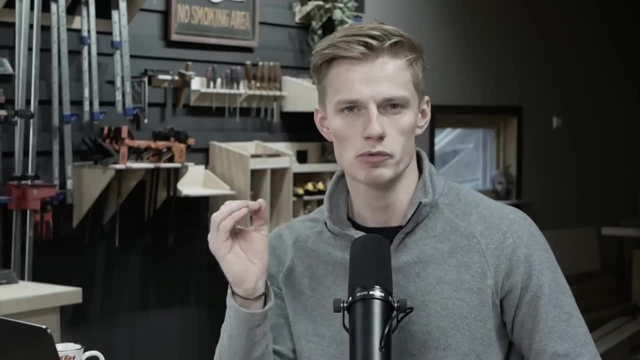 high profit margin and they require a few tools. But first I just want to say something really quick. So when I show you these products, your first instinct is probably going to be: no one would pay for that because it's so easy to make. But you have to remember that most people 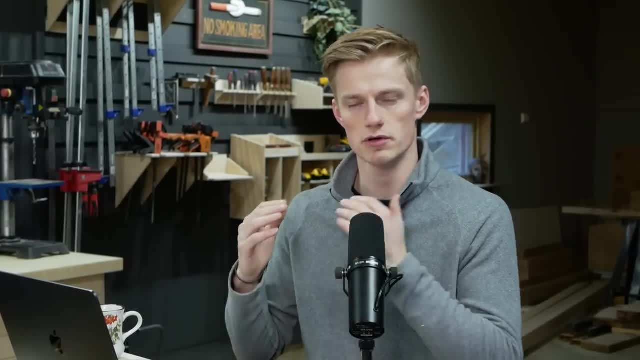 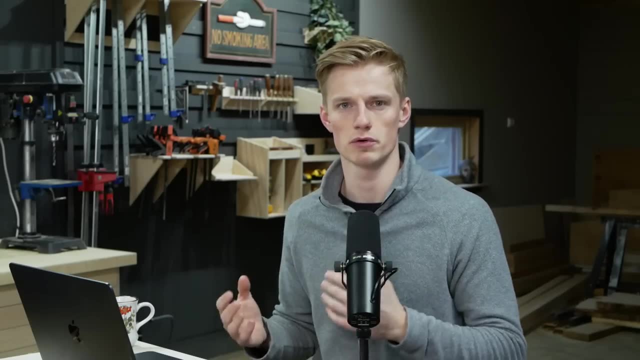 don't think like that, because most people either don't know how to make things or they don't have the time or the space or the tools to make things, So they'd rather pay someone who knows what they're doing to give them the finished product, And so that is why you and I can make money by 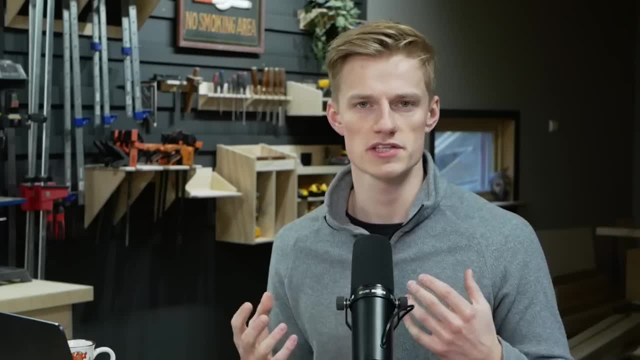 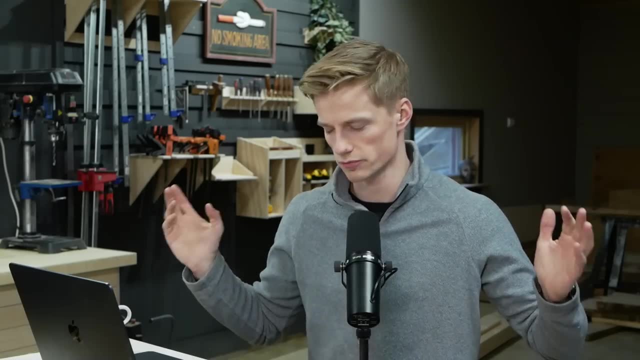 selling easy woodworking projects because they're easy for us but they're not easy for everyone. So number one is a great one. I mean they're all great. To be honest, I wouldn't show you some baloney. This one you can make it from. 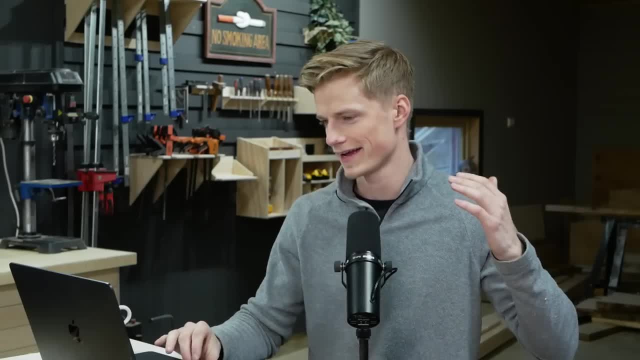 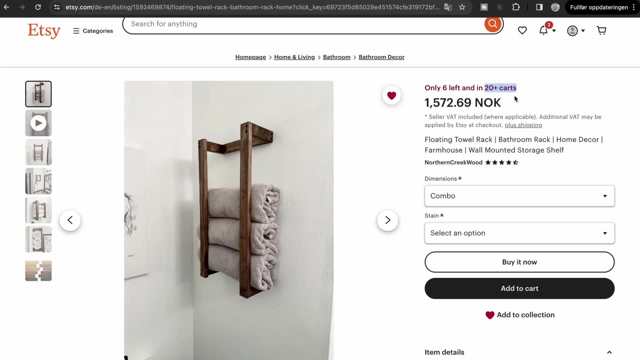 probably just one meter of a two by four And it is the floating towel rack. So looks like this And you can see it's in 20 plus cards. So that means that right now, 20 people have added this to carts and they're either contemplating buying it or they are going to buy it. So they are.